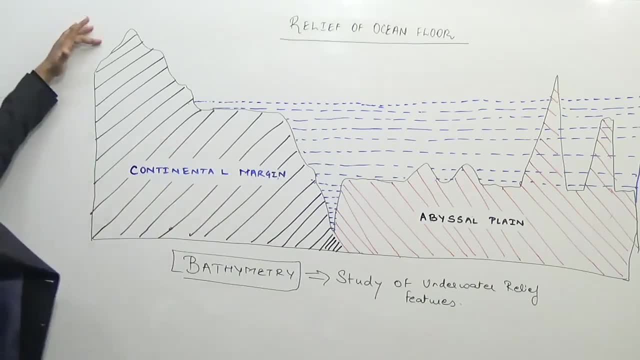 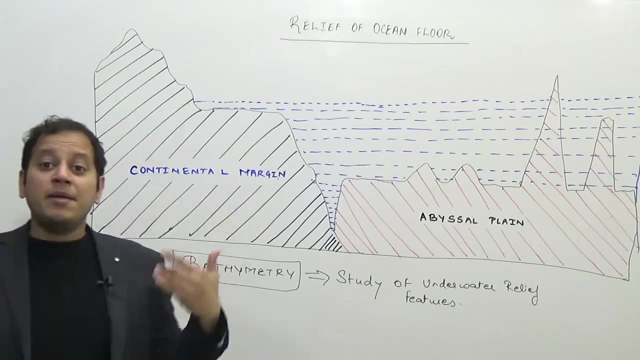 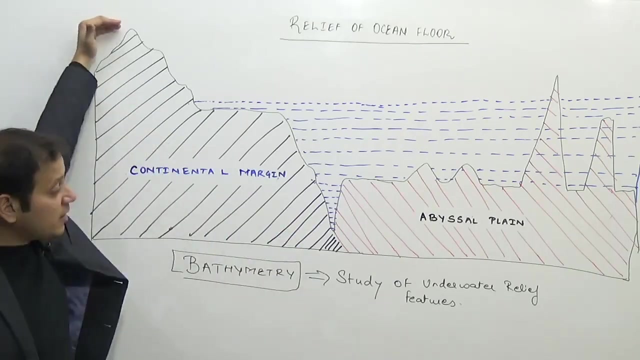 what I have drawn here. what does this diagram show? it shows the height of a mountain. it shows the height of a, maybe a plateau- I cannot show you here because of the limitations of the board. it may be an, sometimes there can be a mountain, sometimes there can be a plain area. so it shows the highest point on the earth and it also 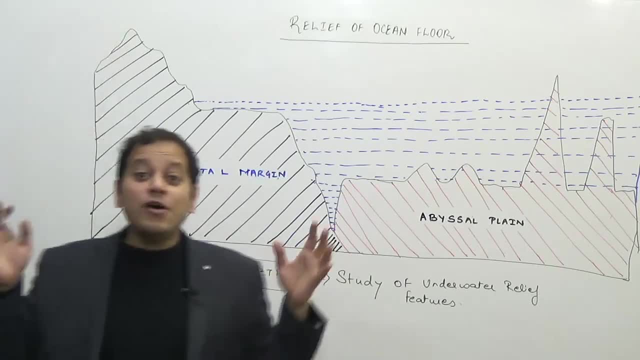 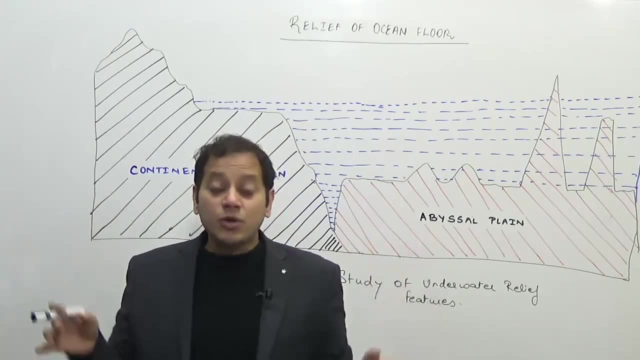 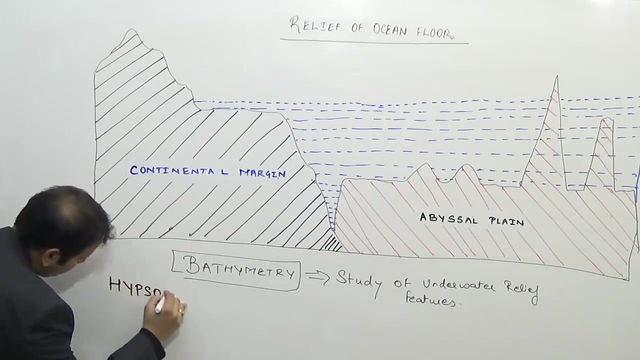 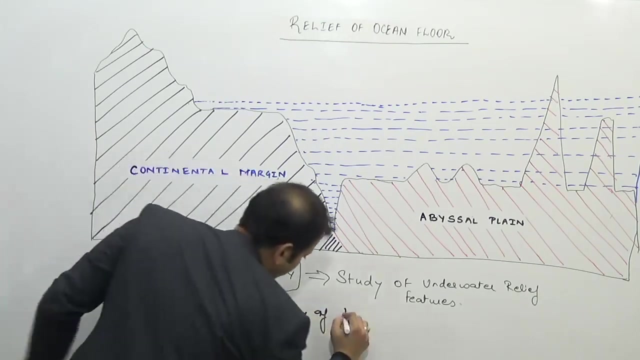 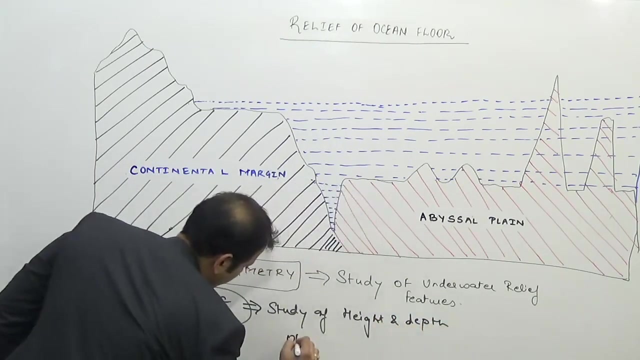 is showing the lowest point of the earth. Such a study of an height of the earth's surface, such a study, comparative study of the height of the earth's surface, is shown with the help of a curve which is known as hypsographic curve. So what is this hypsographic curve? It is study of height and depth of earth's surface. 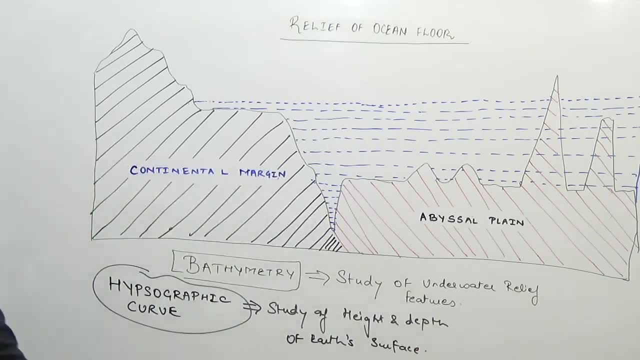 So this hypsographic curve will show you the study of the height and the depth of the earth's surface. So this is a study of an height and depth of the earth's surface. So this is a study of an height and depth of the earth's surface. 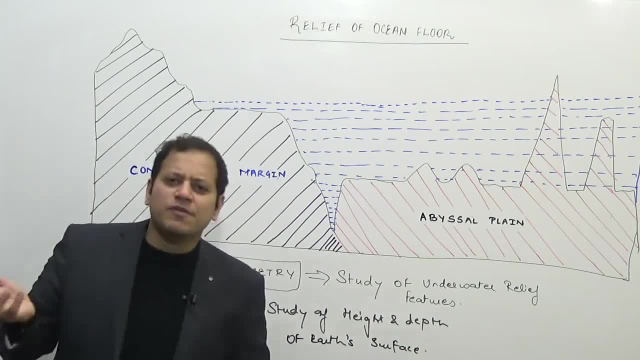 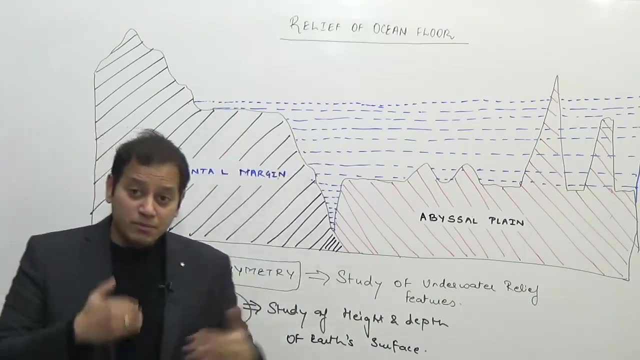 height and the depth of an. a comparative study of the height and the depth of an earth surface bathymetry is the study of underwater relief features. that is, how does the world below, below the water, looks like? now? these are the two concepts which can be asked in the preliminary. 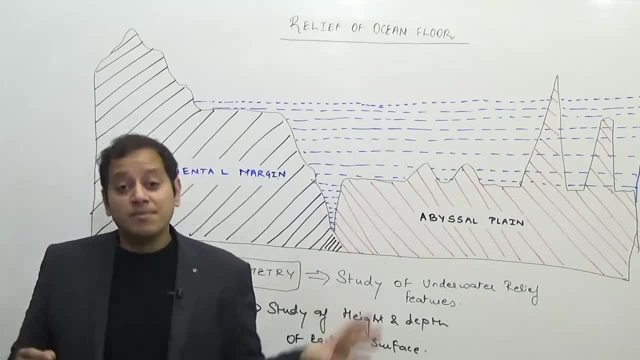 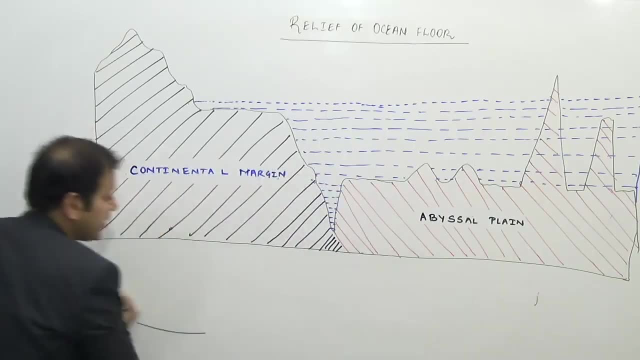 examination. you should not get confused between what is bathymetry and what is an hypsographic curve. now coming to later part, when, if i draw and if you look at the cross-sectional view of an ocean, now this is a continent, this is a part of a continent. obviously, i have shown here in the 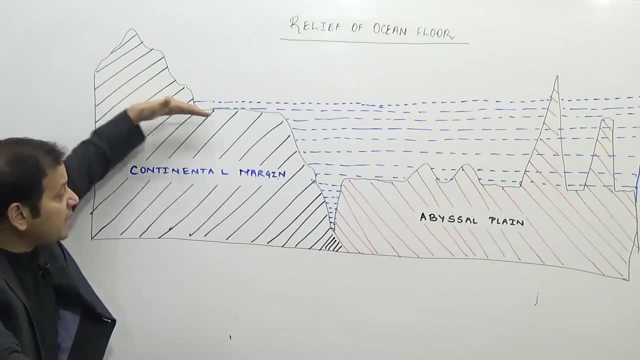 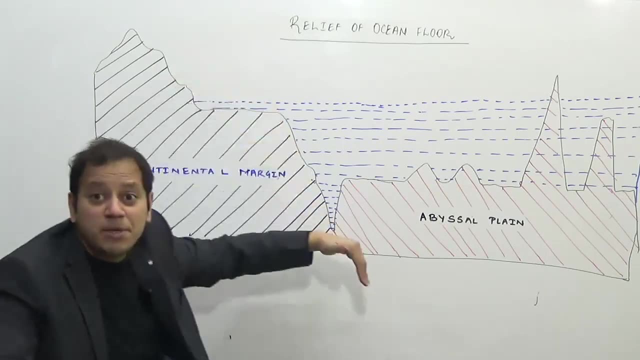 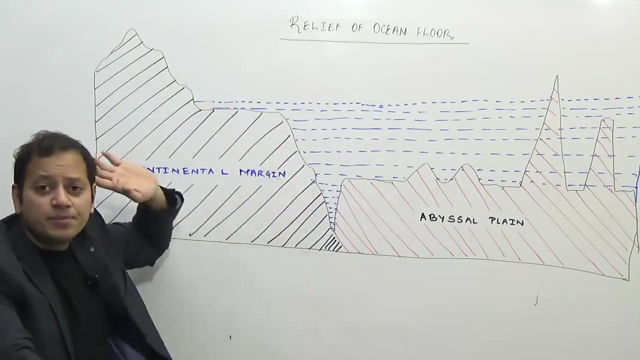 diagram this as a mountain. after that there is a flat terrace like surface on which the water will cover, on which the ocean water covers. after that there is a steeply sloping surface after the ocean terrace and then there is a slightly bulge or slight rise in the ocean surface. 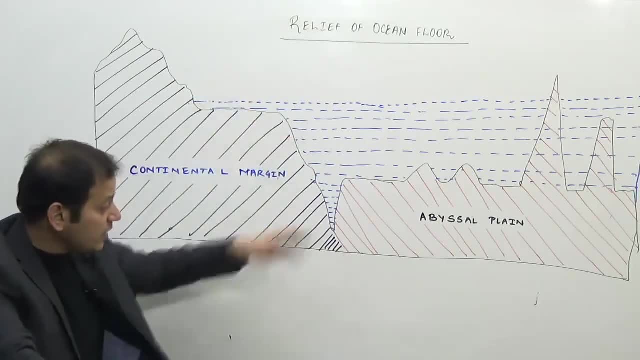 then there is a depth, very high depth, of an, or there is a, we can say a trench, which is of a greater depth. a便 is amäß ain terrace en ang barye. okay, like then, there is a Intro to facts on view治 notorius on the twin axis Asia- oceania. 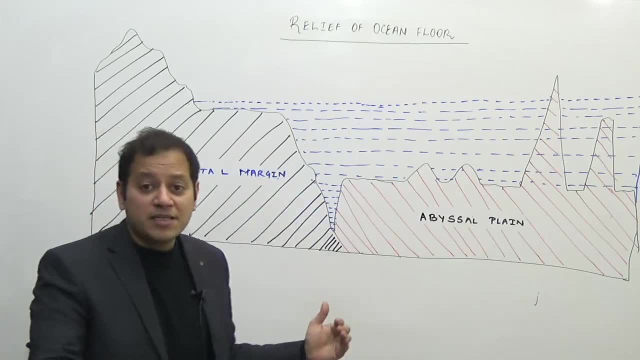 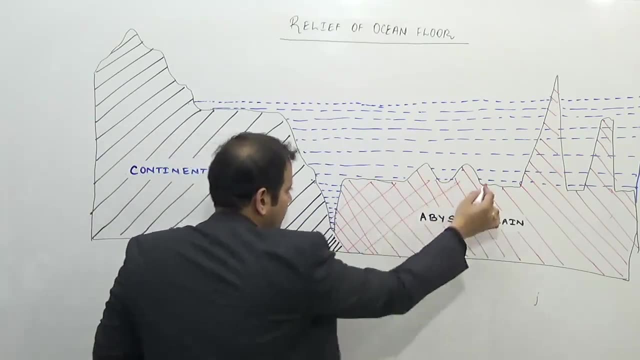 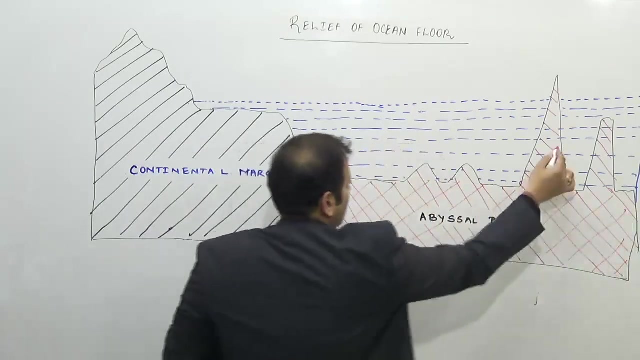 depth in the ocean surface and then the red color part starts. this is reddish in color or this part is having. i have shown you different color because of some concept which will be doing here with the, along with the extra series. now, if you cannot see the color different, because 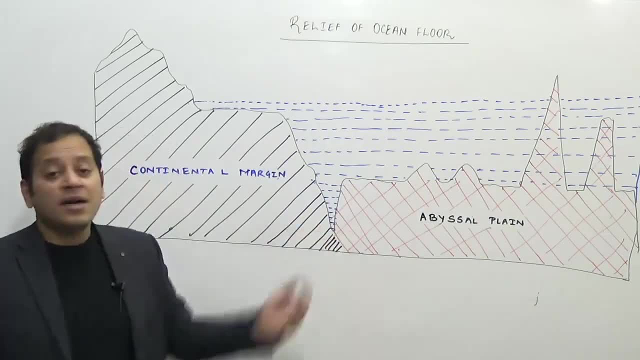 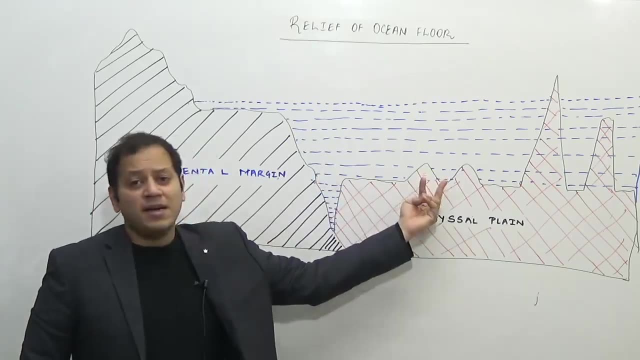 one is reddish in color, one is bluish in color. we, i have marked even shaded it differently. so after that starts a different part, which is which is having up to parallel mountains, which is having an isolated single mountain and also having a single mountain on which is a more or 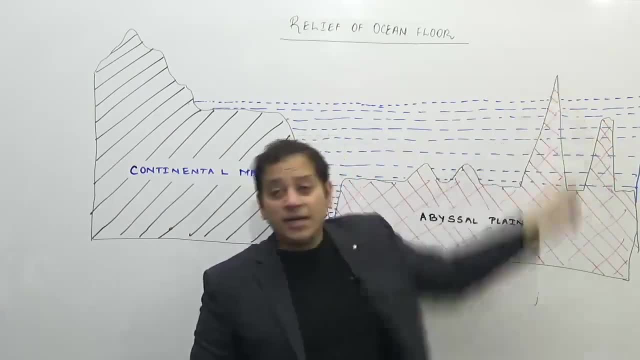 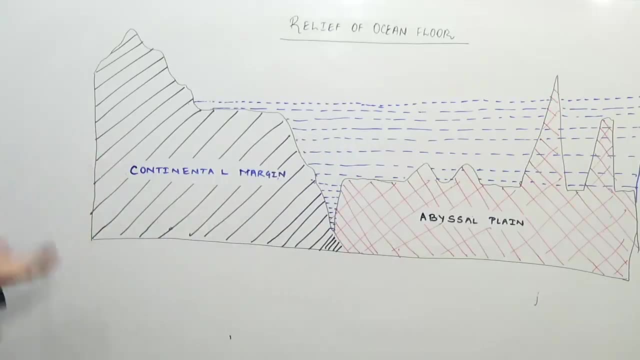 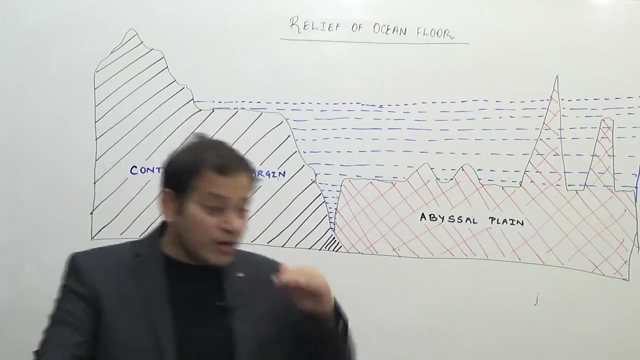 less a flat top mountain. it is not as pointed as this mountain. so this is what is an ocean relief feature. now, what are these features which i have drawn in the diagram? the first feature, which is a flat terrace like feature, is what? what is the terrace like, or what is the flat? 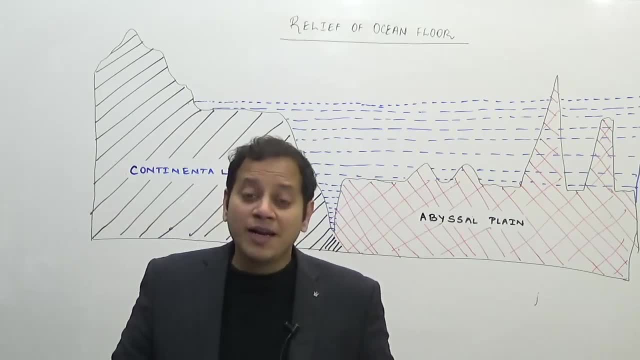 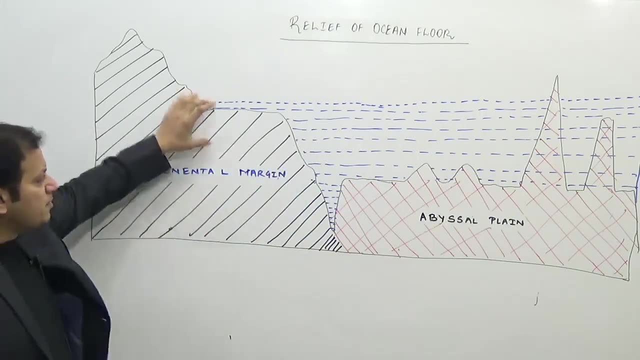 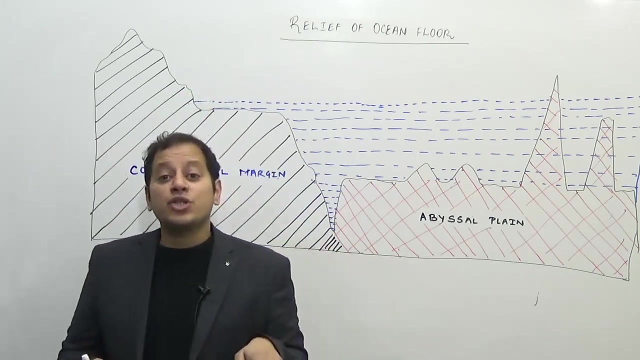 feature in your cupboard, what you call as shelf of the cupboards. after that, now you see here this shelf part, or this part till here, black in color, is an extension of a continent, or it is a part of a continent which is below the ocean water. therefore, this area is known as an continental. 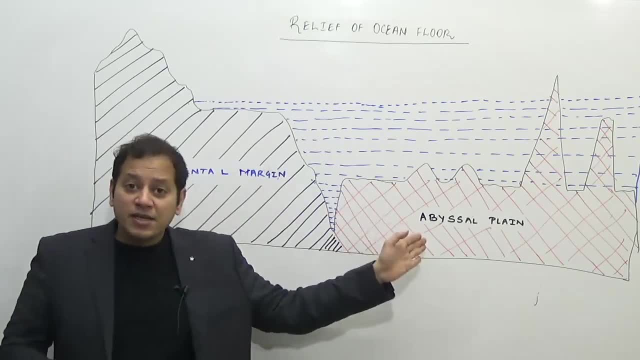 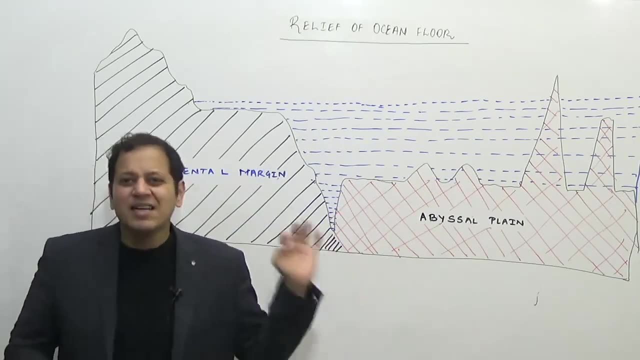 margin. while this is a part, the reddish in color, the other part is made up of flat ocean floor. it is made up of an ocean floor floor and it has some of the other relief features. now this part is known as a deep sea plane. it is 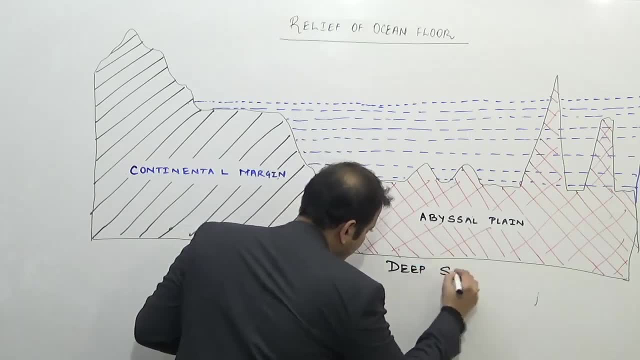 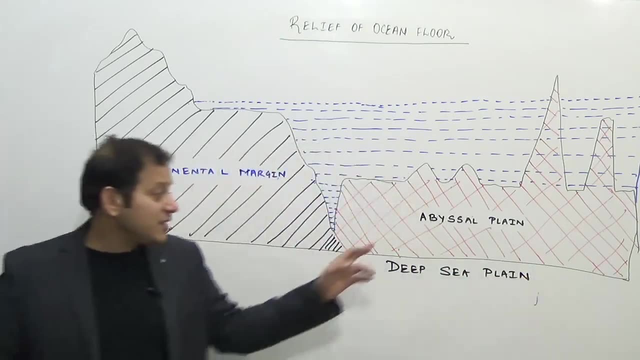 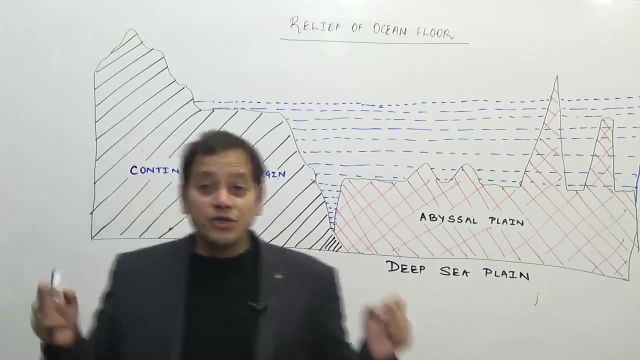 known as deep sea plane, or it is known, in geographical language, as abyssal plane. so what is this abyssal plane? this abyssal plane is made up of ocean floor, while the continental margins are made up of continental floor. now, that is why i said you will require some part of geomorphology. 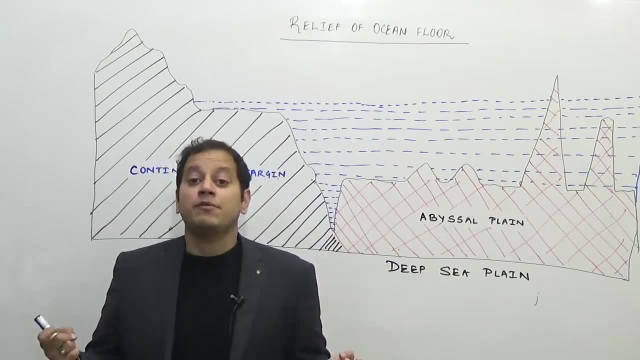 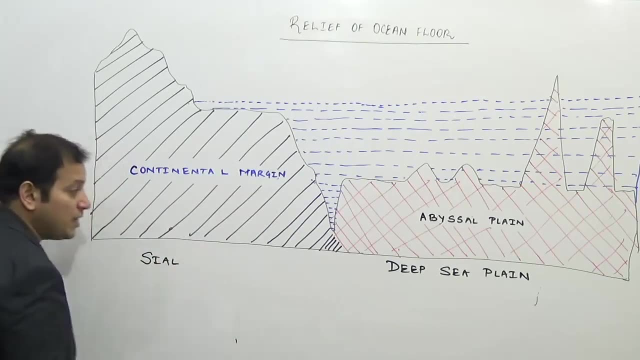 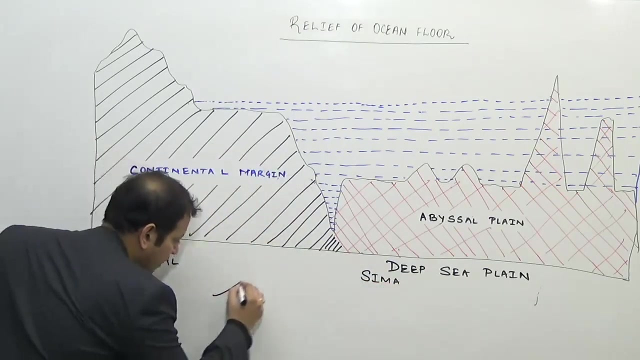 if you remember your lectures, what are the continents made up of? the continents are made up of a concept which we studied, known as seal, while the oceans are made up of a concept which we studied, known as sema. or, if we try to show it, if i try to show it in a diagram, this is how: 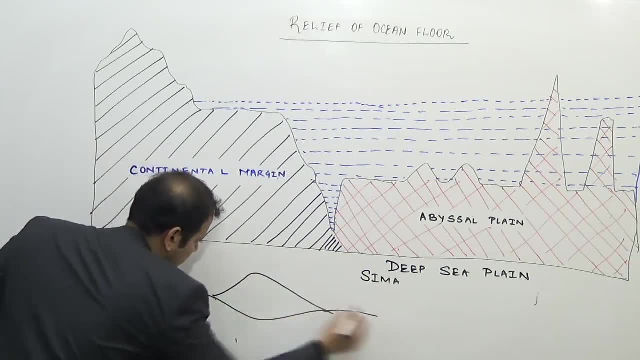 the continents are made up of and this is how the oceans are made up of. so the topper part is seal, while the lower part is sema. this is a sema, and here there is a covering of an water body. this is what we have studied in the 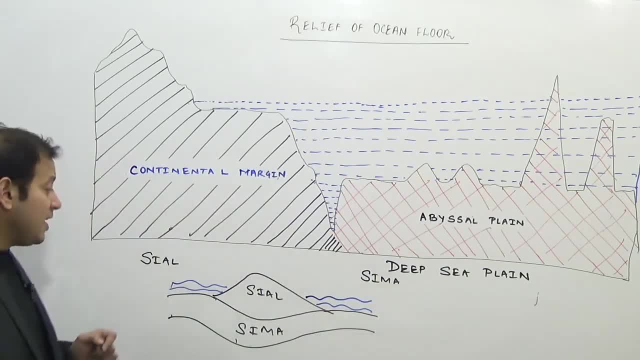 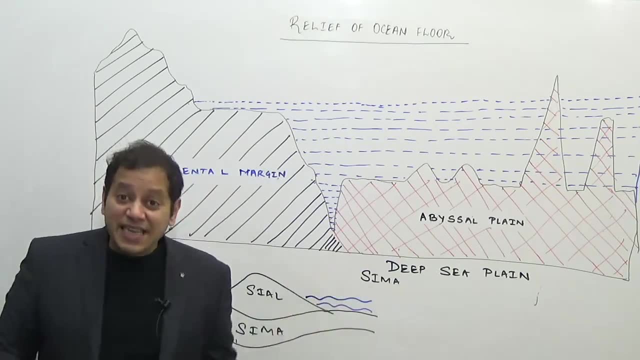 geomorphology lectures. now, what is the seal? seal is made up of silica and aluminum materials, while sema, which is denser, is made up of silica and magnesium minerals. the seal is mostly composed of granite rocks, so the continental margins are mostly made up of granite, while the oceanic margin 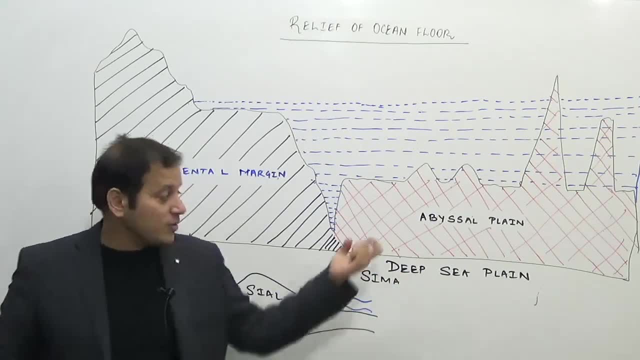 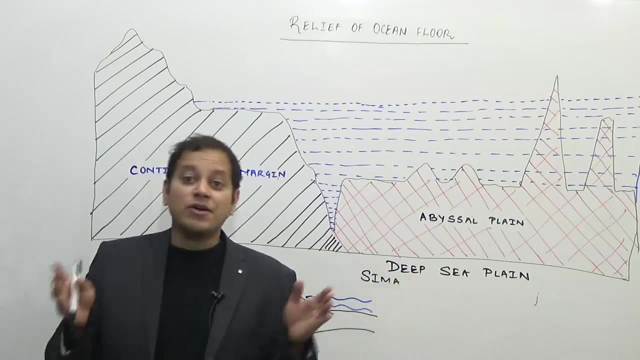 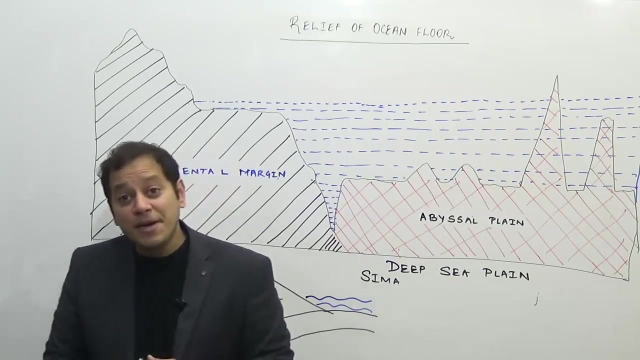 or sema, is made up of basalt rock. so this is what is made up of basalt. big sense basalt is denser than the granite because of the dominance of iron and isla. basalt rock is black or darker in color as compared to the whiter or lighter granite rocks. so we can say: 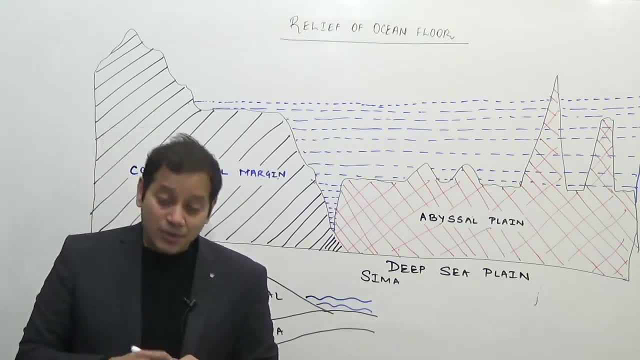 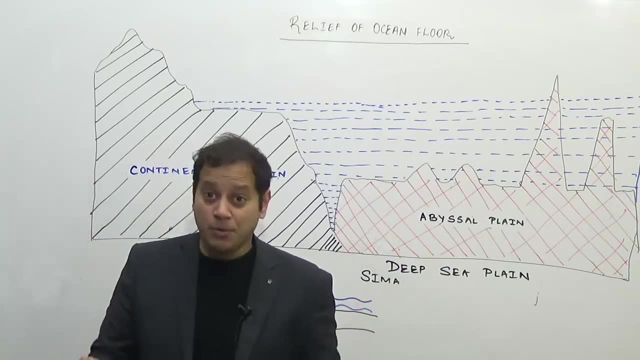 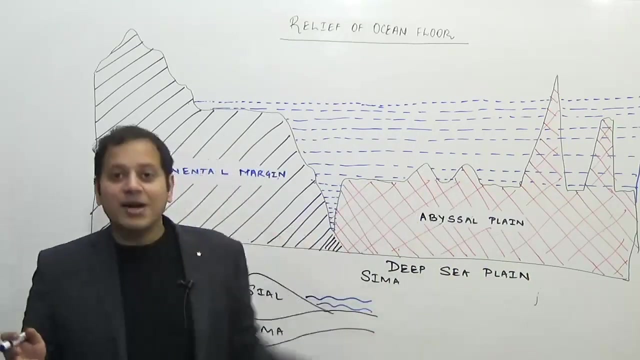 that the continents are lighter than the denser oceans. the oceans are dense and therefore we can say, like a conveyor belt on the airport, continents are floating on the oceans. how does the conveyor belt function? the belt goes round and round and your luggage comes on the belt, so you can see. 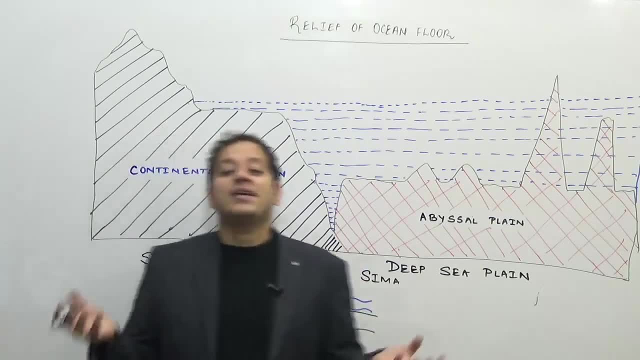 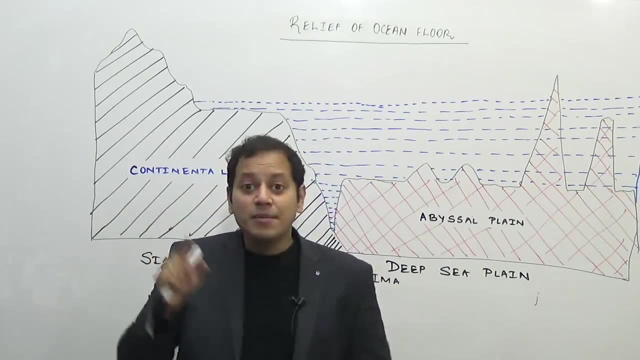 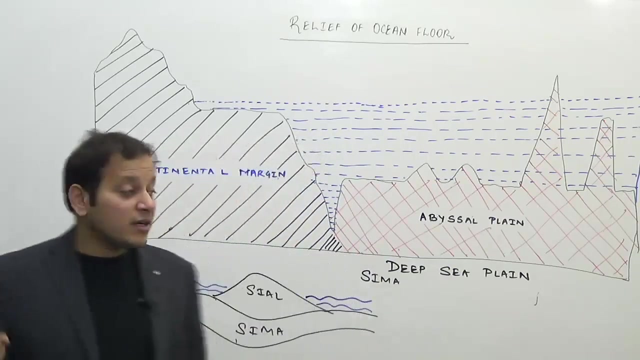 so consider your luggage as a continent and the belt as an ocean. so the belt goes below some. that belt is like a conveyor belt: it goes below and then again reappears, but your luggage keeps on moving. that is how the plate tectonics is explained. like a conveyor belt, the earth functions now you. 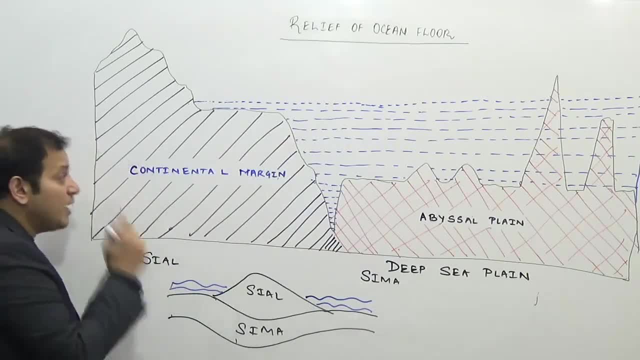 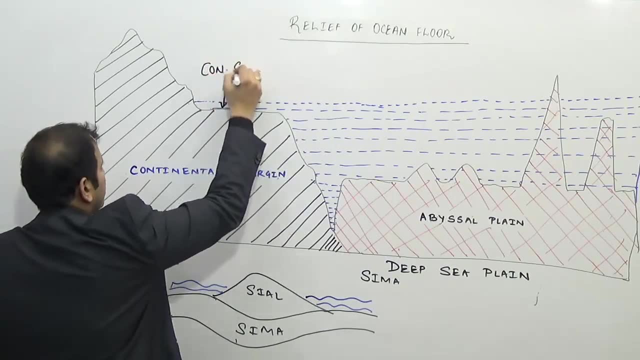 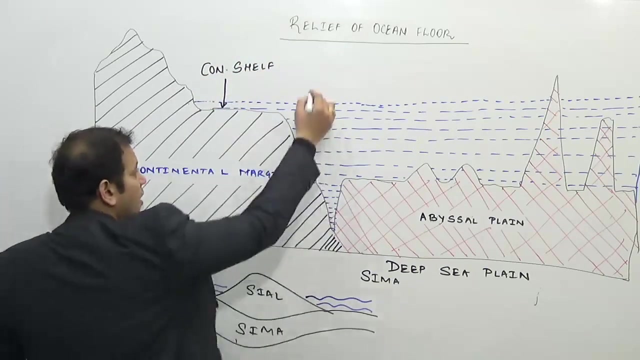 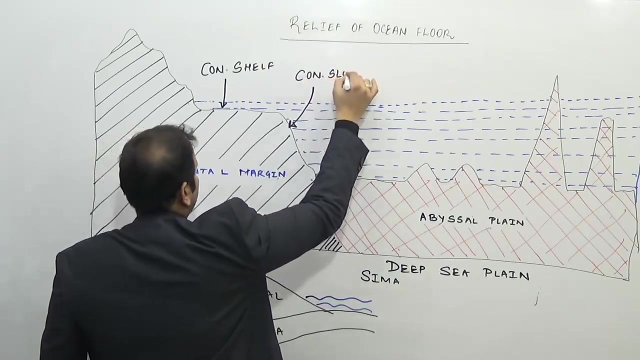 see the continental margins, which is made up of seal, can be further divided into flat terrace, like feature, which is known as an continental shelf. a steeply sloping surface along after the end of a continental shelf is known as a continental slope. is known as a continental slope now, because see what does this. 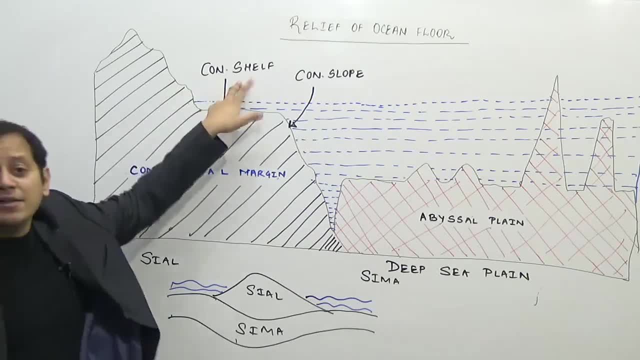 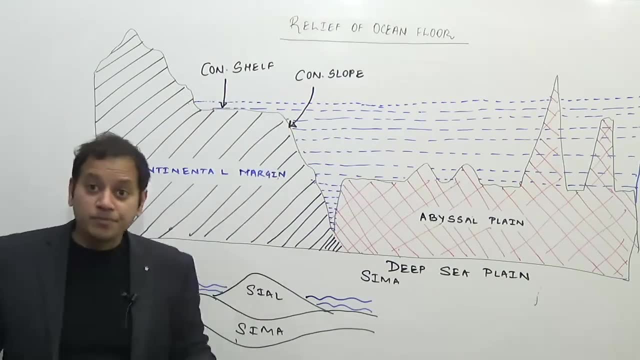 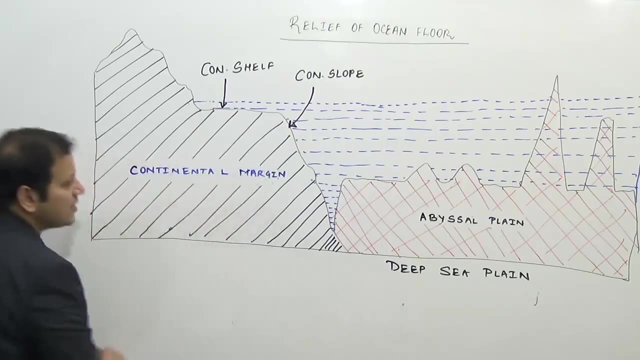 c? o? n means. it means continental shelf either. space is not there to write the entire word, so i hope that you understand it. continental shelf, continental slope, at at the end of the continental slope and the Douglas slightly rising feature- there isn't slightly rising, are slightly uploaded or slightly bunch he. 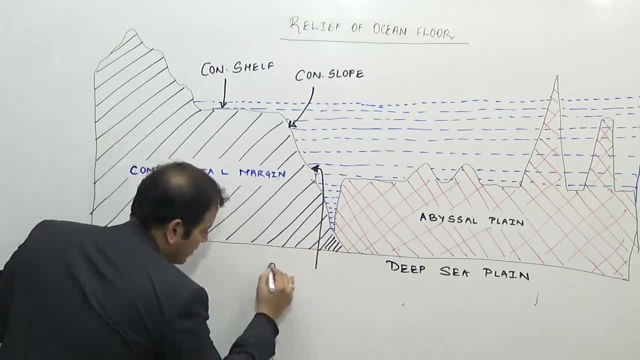 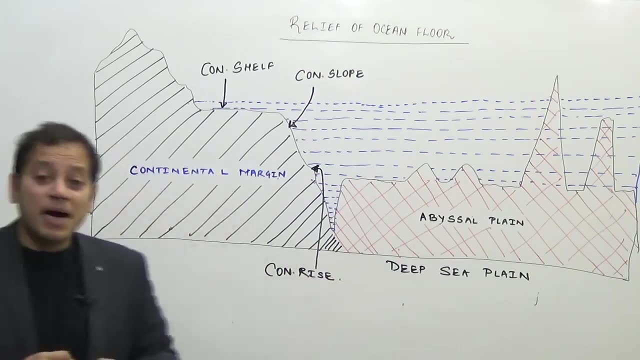 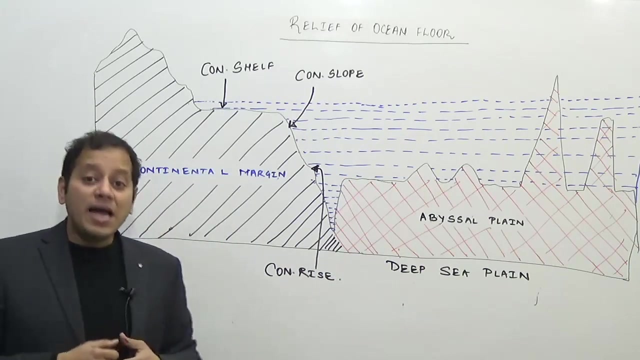 changed. it is known that continental range, which is known as an continental, so the continental parts are made a pair of continental shelf, continental slope, and a continental rise way, The oceanic parts or the abyssal plain, which is the most dominant feature of the ocean. 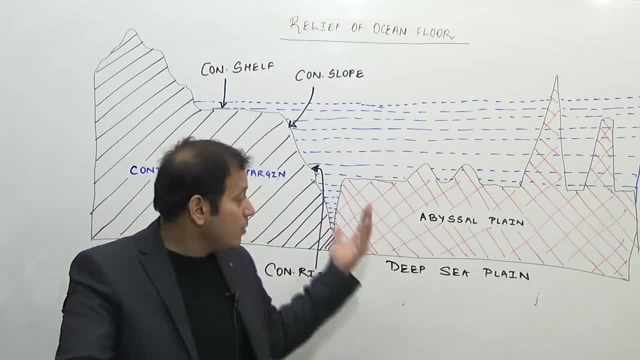 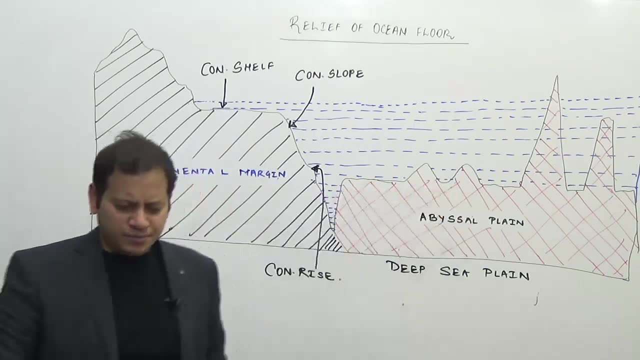 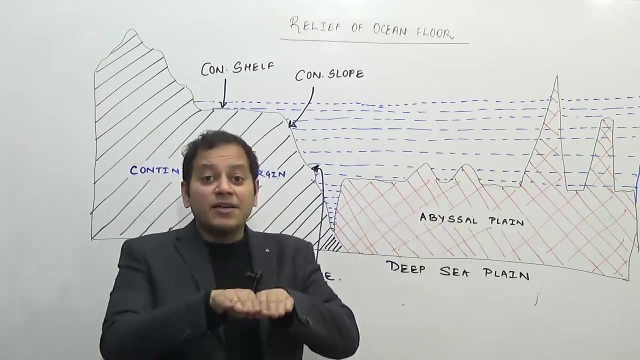 which is not visible to us human eyes, which is very deep, more than 3000 meters deep inside the oceans, is made up of two parallel mountains. Again, apply your geomorphology feature: These parallel mountains reflect or these parallel mountains are nothing but the divergent. 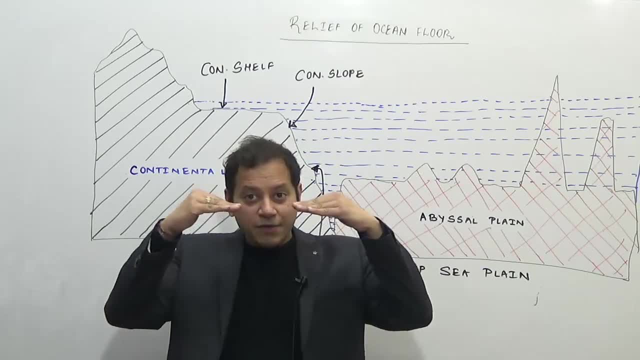 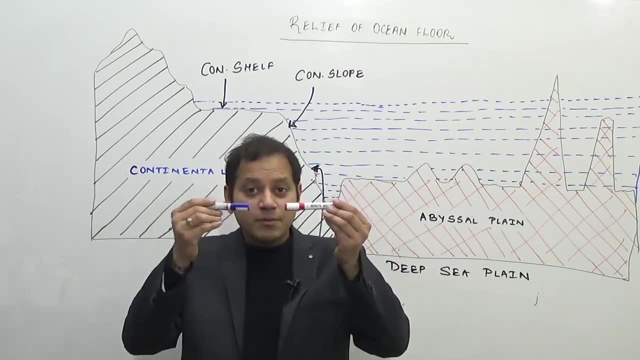 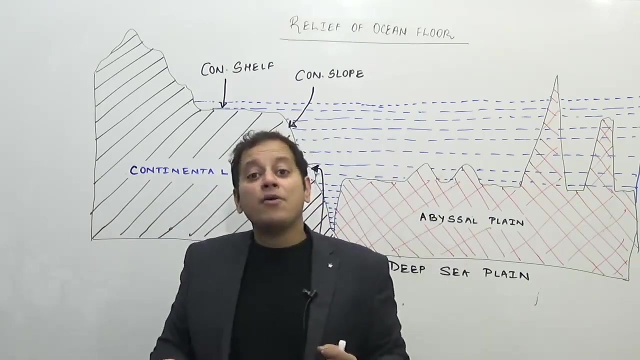 plate boundaries where the two plates are moving away from each other. Because the two plates are moving away from each other, the two oceanic plates are moving away from each other. the magma, or lava, comes out as it comes into contact with the above. 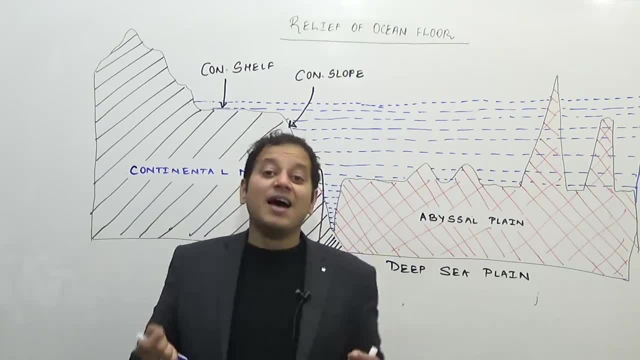 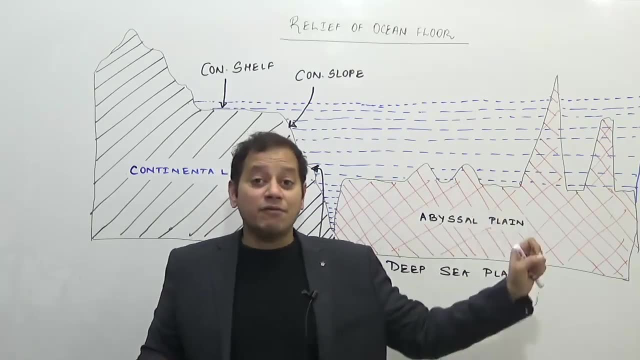 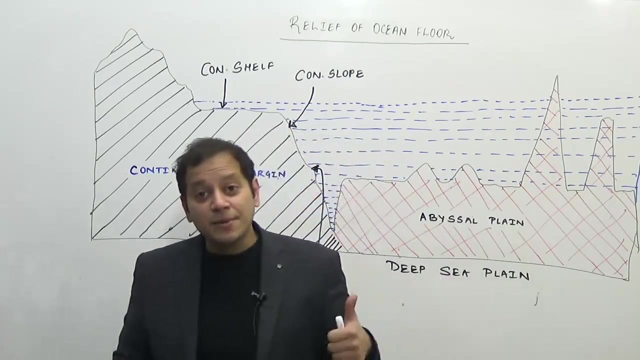 water, it solidifies before flowing for a large distance and hence, if you know, the parallel mountains known as mid-oceanic ridges are formed. For further clarification, You can watch the lectures on geomorphology, the seafloor spreading theory. I think it is. 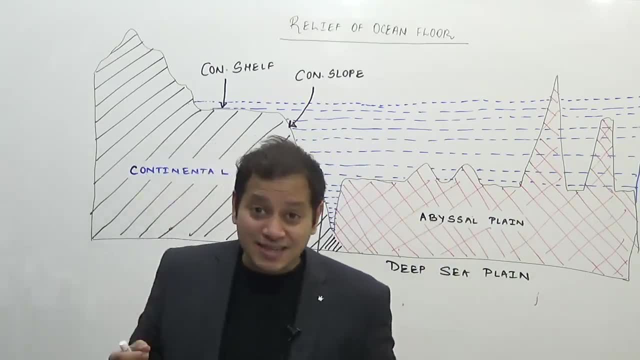 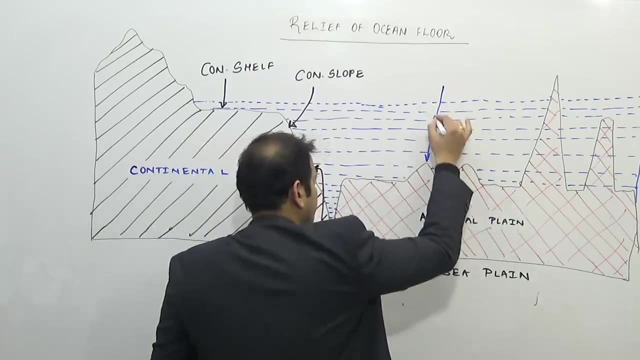 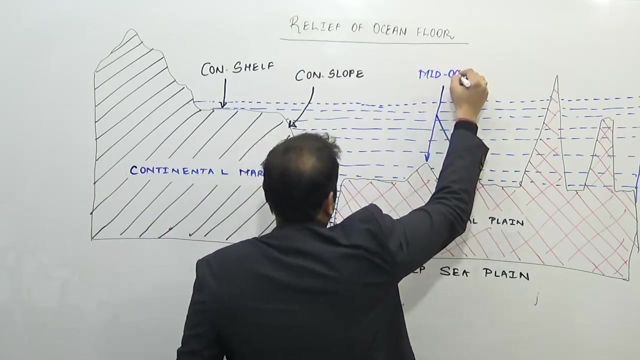 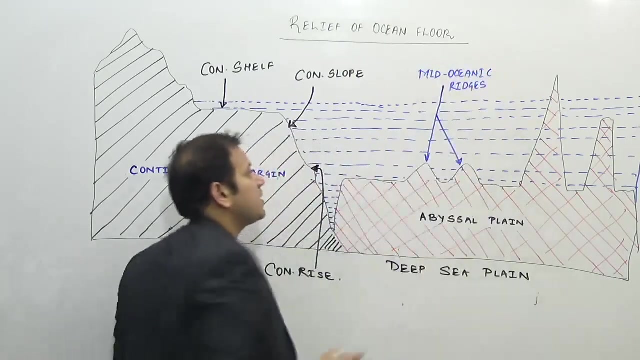 in more of an animated lecture so you will be better able to understand it. So what are these? These are nothing but mid-oceanic ridges. These are nothing but mid-oceanic ridges. These are mid-oceanic ridges. 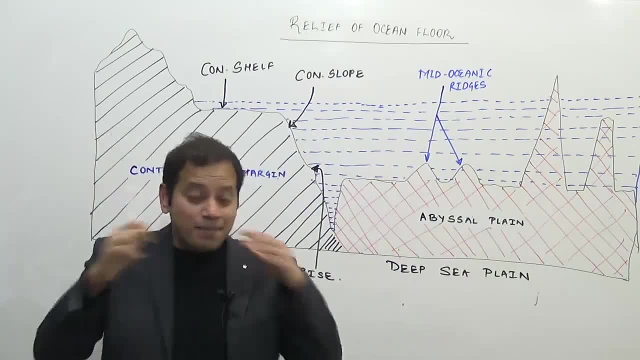 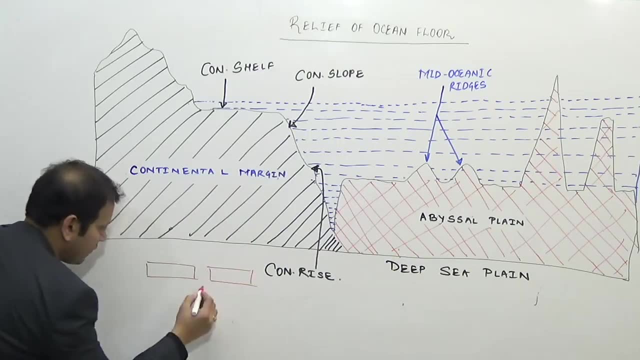 Why two? Because, as the plate separates from both the sides, there is one plate which is going in the opposite direction to the other plate. Therefore, the magma comes, gets solidified, the magma comes and gets solidified, forming a parallel mountain system. 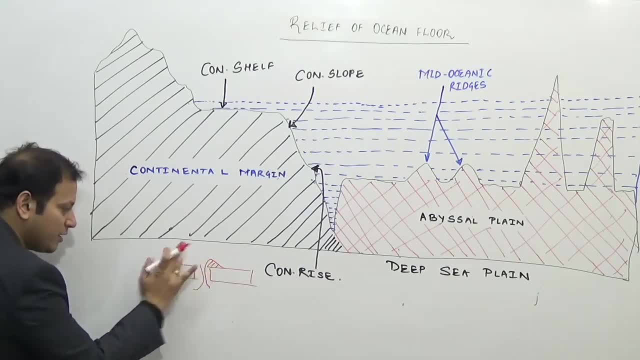 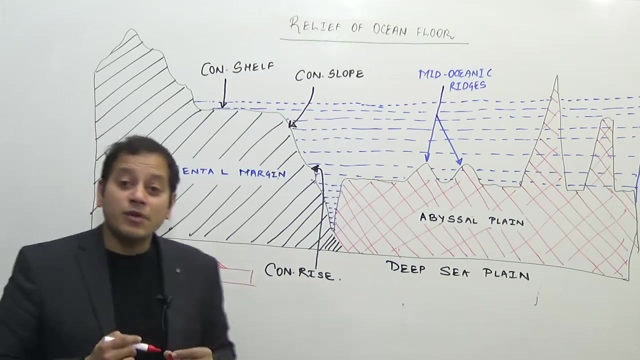 As the plate moves further, this older mountain will be displaced or placed to the other side and its place will be taken. This place will be taken by new magma and lava to get again solidified. So this is how the mid-oceanic ridges will be formed and therefore, because they are 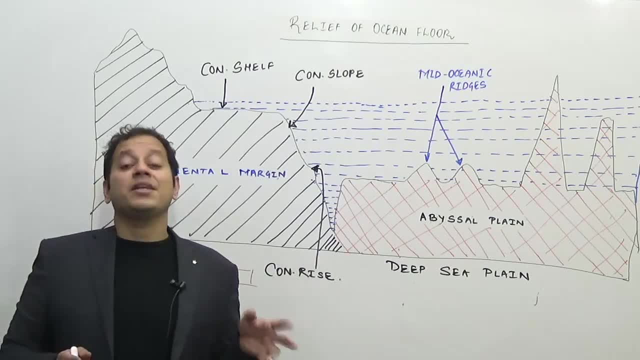 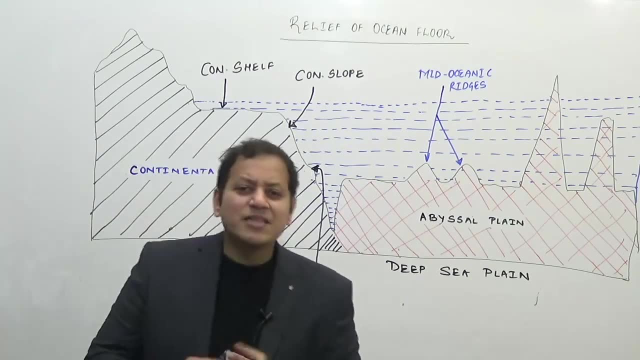 parallel to each other. we are not calling them mountains, we are calling them mid-oceanic ridges. Now what, from the exam point of view, question can be described? The relief features of an ocean? or from the prelim points of view, they can ask you to. 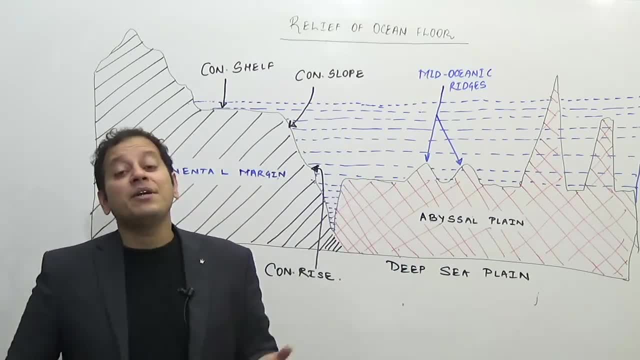 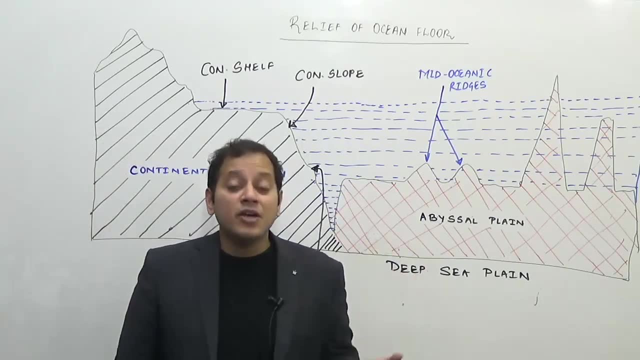 describe the releases: The mid-ocean. What is the name of a mid-oceanic ridge in Atlantic Ocean? What is the name of a mid-oceanic ridge in the Indian Ocean, which obviously we are going to cover it in the class? 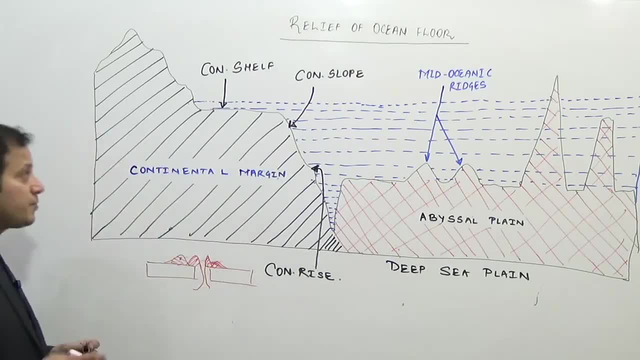 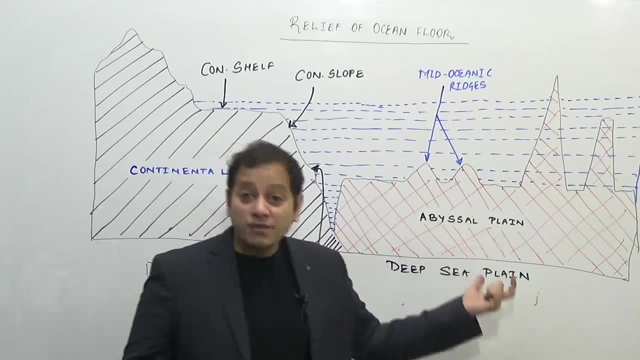 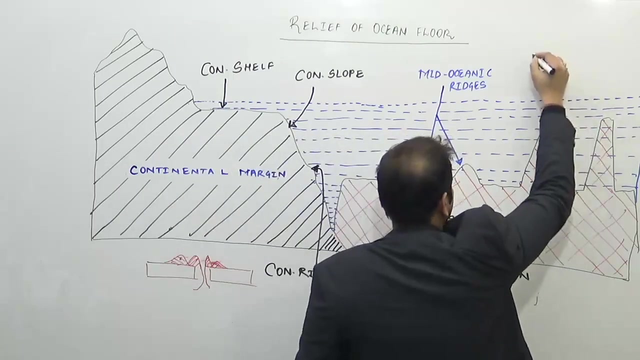 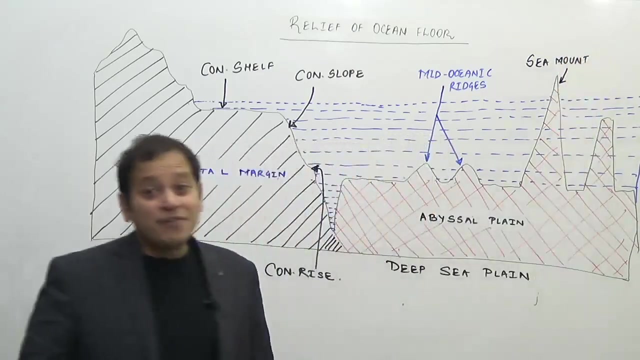 So these are the mid-oceanic ridges. Now, after that, an isolated mountain which rises abruptly from the ocean floor, from the deep ocean floor, is known as a sea mount. Why this sea mount rises, If you remember the concept of a hot spot in the geomorphology lectures. 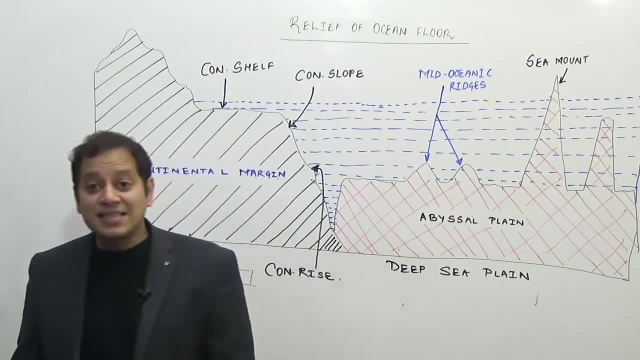 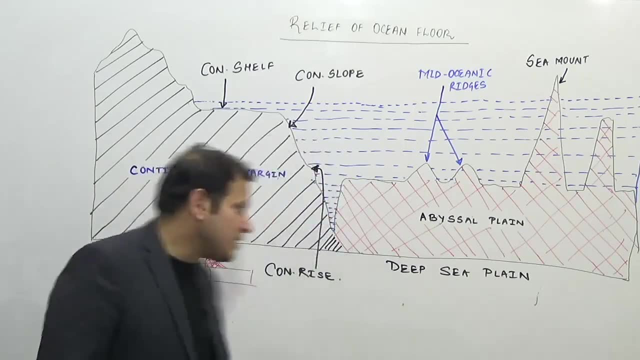 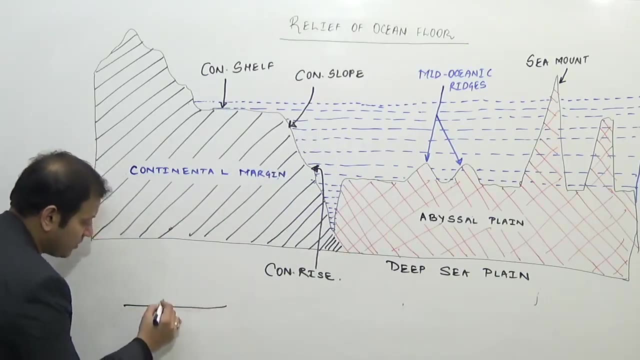 that is, the areas which are having less, which are weaker sections of the earth and therefore volcano continuously erupts from this region and, as a result, the if in the, on the ocean floor, the volcano erupts and keeps building a mountain. 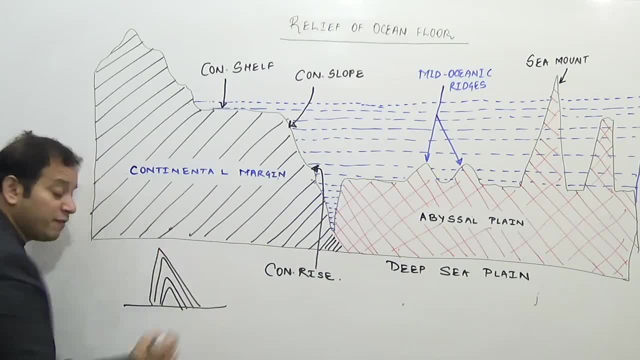 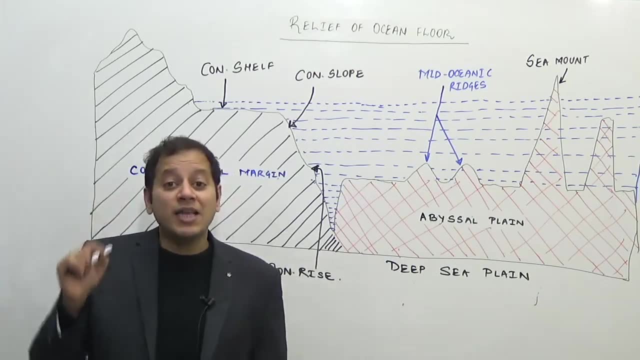 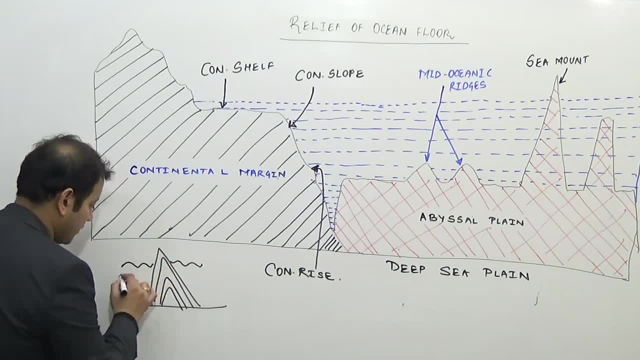 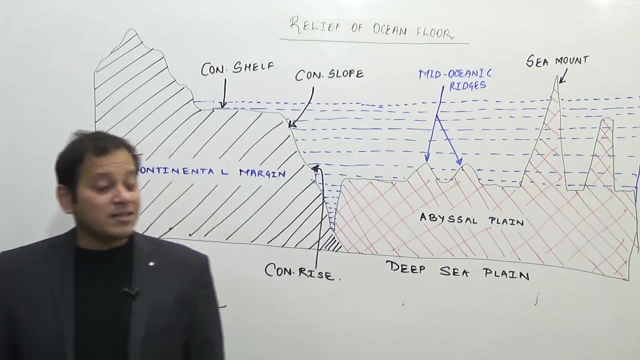 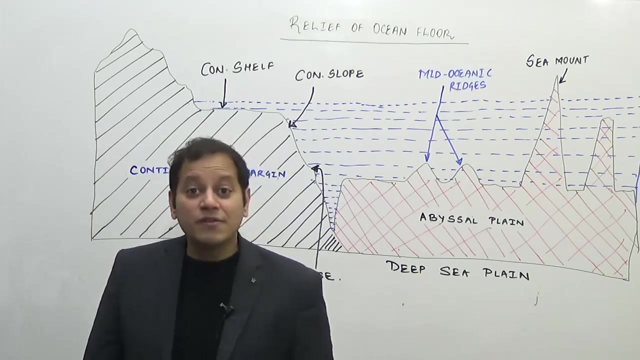 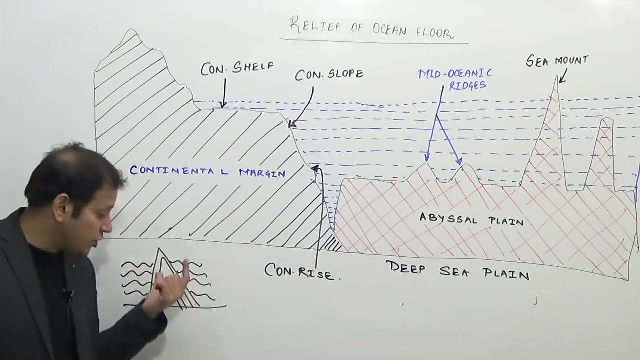 So, over the period, a mountain keeps building and if its height is more than 1000 meters, then it is a mountain. what are these examples of a seamount now? lastly, the flat topped seamount. now this is a seamount. obviously it is washed by water because if you now again geomorphology, weathering and erosion, water is the most powerful agent of weathering and erosion, so the water causes large amount of weathering, and erosion means it removes the relief features. the relief features which are of greater height will be made flat by the different agents of erosion, out of which water and oceanic water. 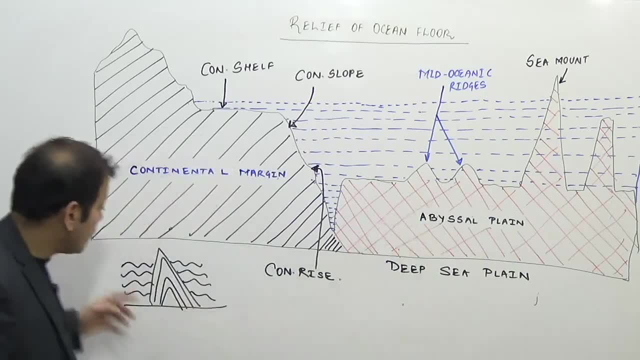 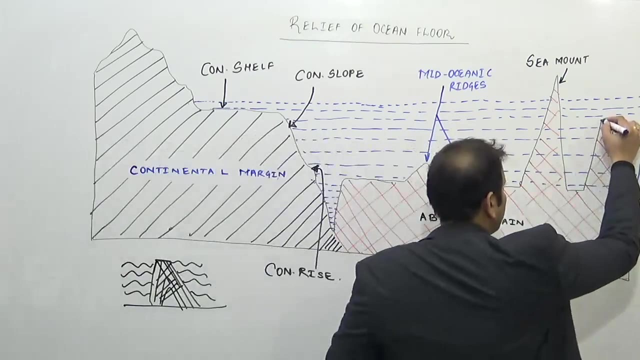 in the form of waves, are the powerful agents. so, over the period of time, this seamount will be eroded and the mountain will become a flat topped mountain. such a flat topped mountain seamount is are known as they are known as guillots. these are known as guillots. 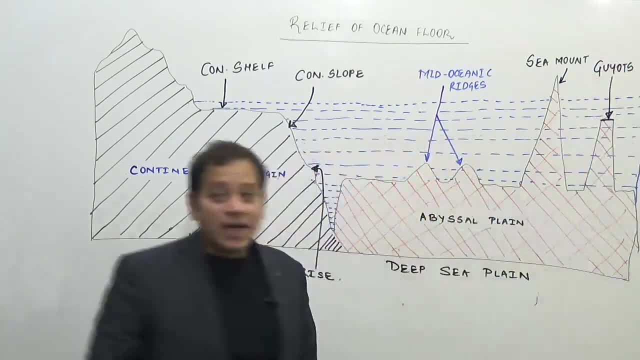 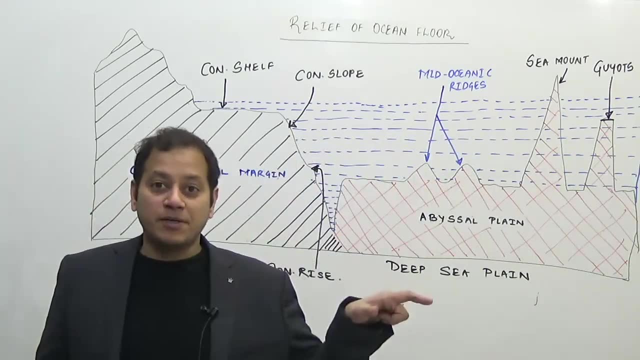 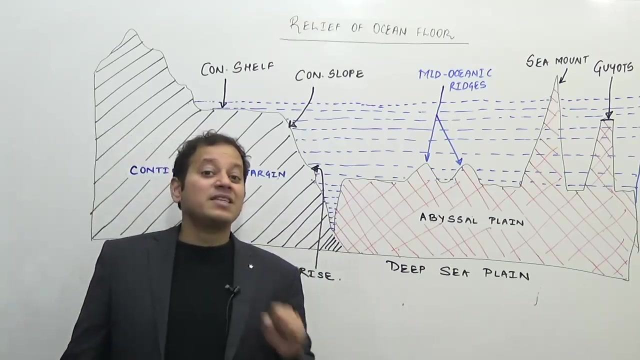 you. these are known as guillots, g-u-y-o-t-s. so what are guillots? remember flat topped. once the guillot comes in your, if you hear the word guillot, you should remember flat topped seamount. lastly, you can see some of the deepest part of the oceans which are still unaccessible to us, which are 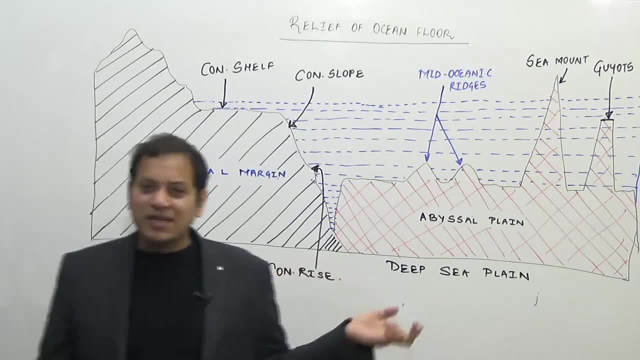 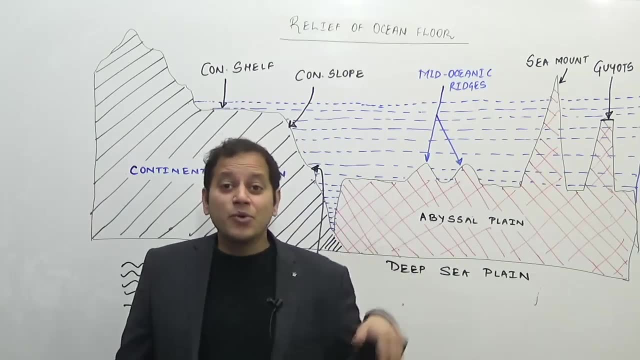 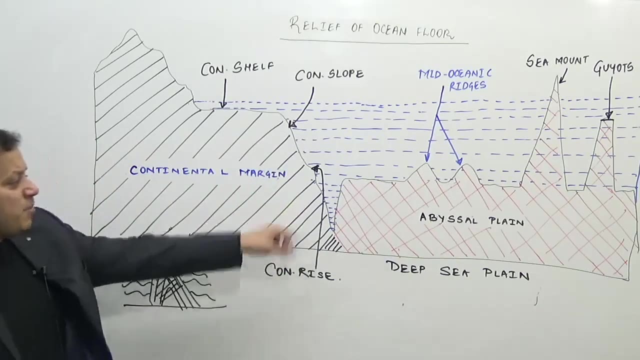 still unaccessible with the help of modern technology. in fact, the maker of a titanic or maker of the movie avatar is the only person who has tried to go inside the deepest part of the ocean, maybe for his movie or something. so, this deepest part of the oceans which reflect what do 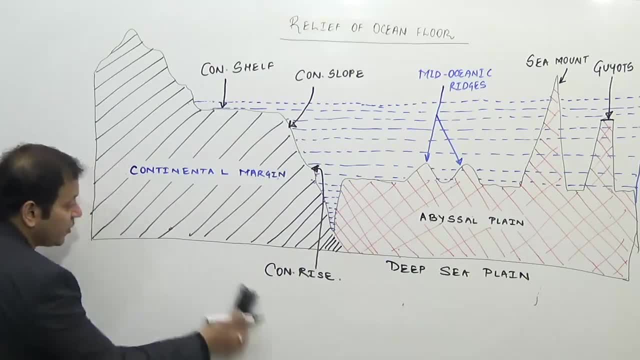 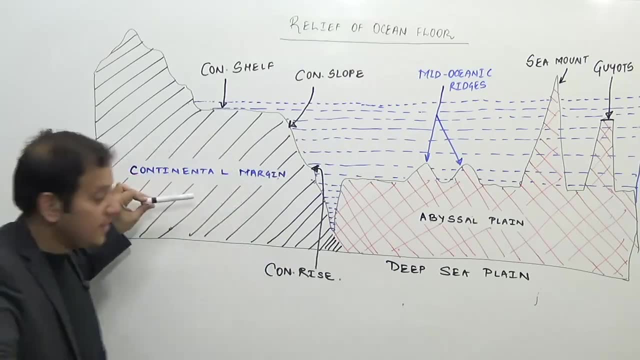 they reflect again your geomorphology plate, tectonics lecture. what do they reflect? they reflect two plates. this is an continental plate, while this is an oceanic plate. what happens? the continental and oceanic plate come in two different places. one is an oceanic plate and the other is an. 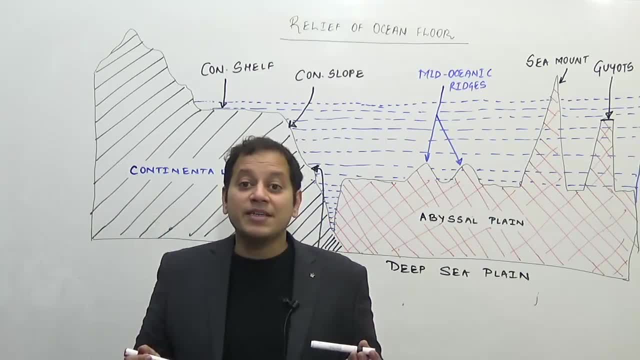 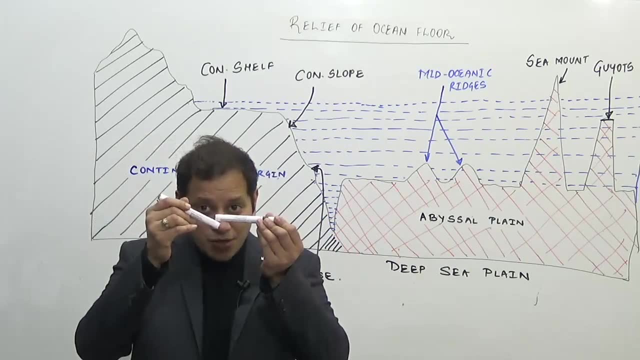 near each other at a boundary which is known as a destructive boundary. at the destructive boundary, because the oceanic plate is heavier, it goes below the continental plate, if you remember, and resulting into formation of an fold mountain, see happy- while downwards, downwards, the oceanic plate goes below. 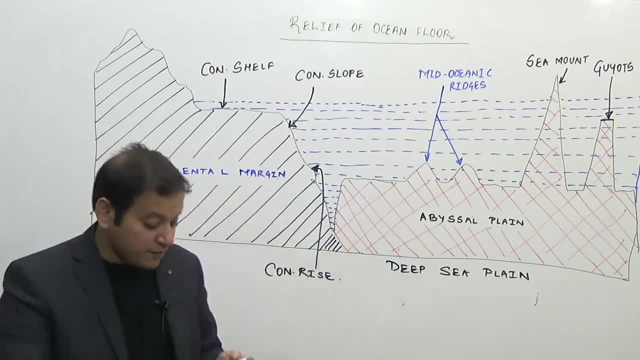 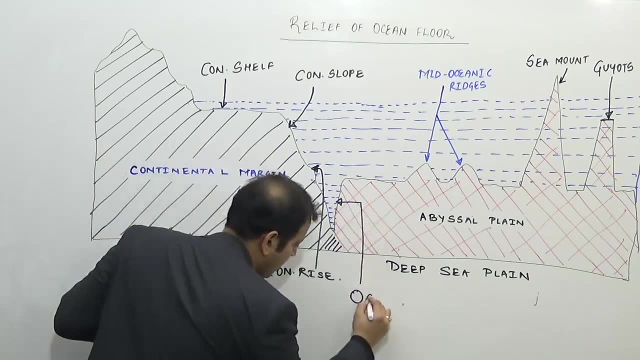 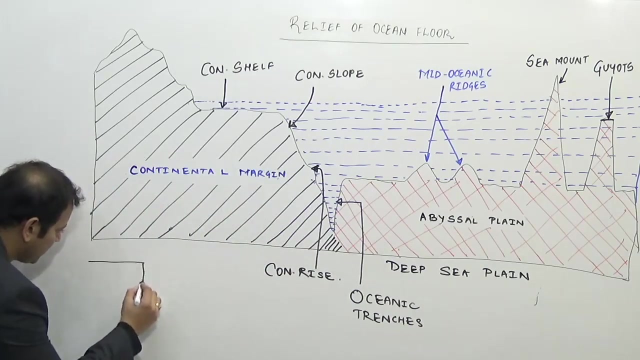 and this gap is what is reflected on the surface of the earth as oceanic trenches. these are oceanic trenches. these are oceanic trenches. how are they formed? refer your geomorphology lecture and also I will give a short explanation. if this is a continental boundary, continental plate, and, on other hand, if 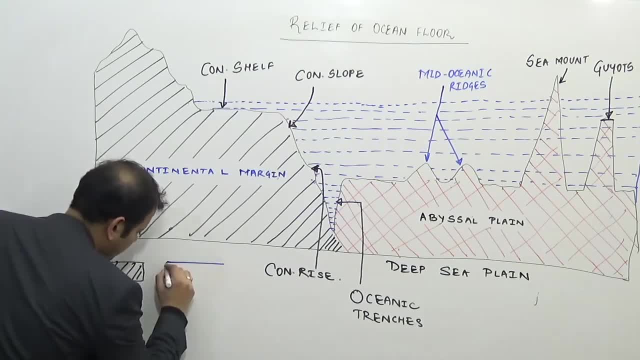 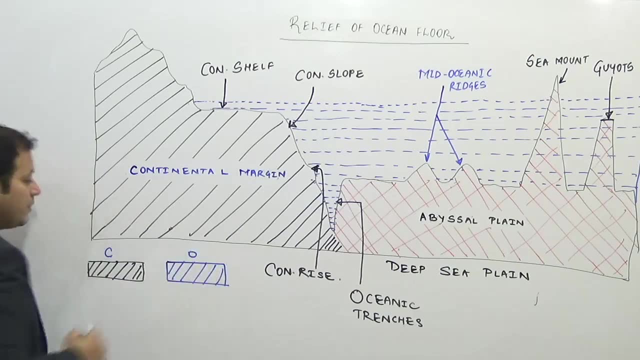 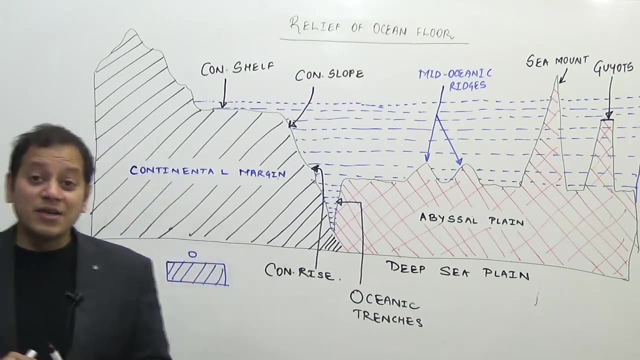 this is an oceanic plate. if this is an oceanic plate, this is continent. this is an oceanic plate. now, by CL and SEMA, we know that the continental plates are heavier than the oceanic plates and therefore, the continental plates being heavier than the oceanic plates, it will give the quantity: oceanic plate. sorry, the continent of continental plates are lighter than the oceanic plates. that means the oceanic plates are denser than the continental plates. so when this to collide, what happens first is the sediments which are there. on this, both the plates are converted. 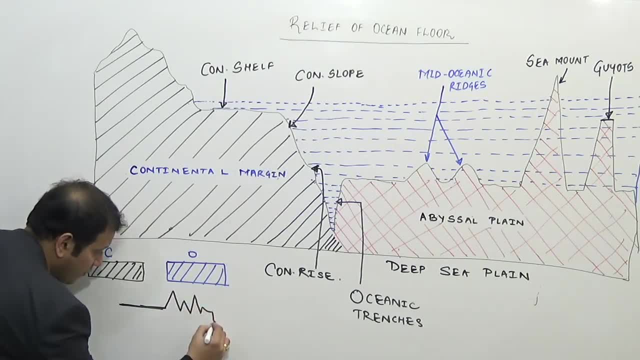 are wrinkled, are folded to give rise to the fold mountains, because there is high amount of folding of the plates giving rise to the fold mountains. on other hand, the oceanic plate goes below the continental plate. on other hand, the oceanic plate goes below the continental plate. 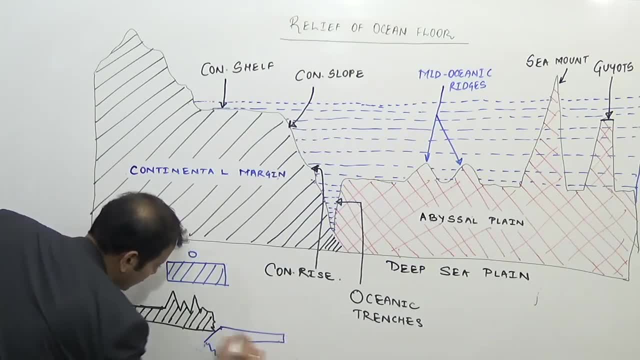 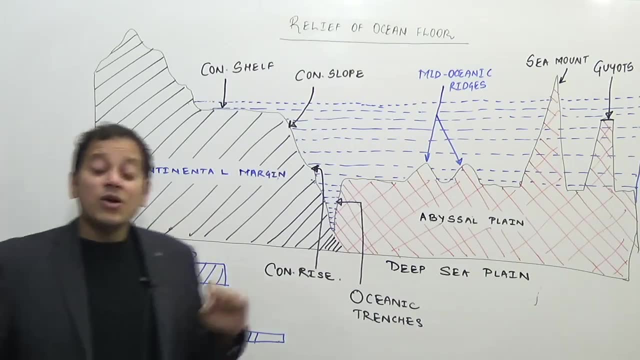 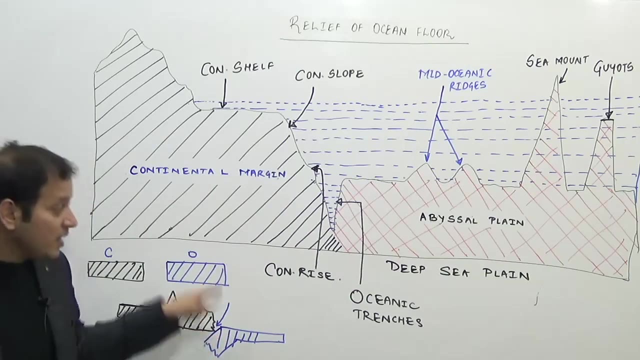 so this is a boundary. this part of the earth's surface is known as the part where the continental plate rises above or the oceanic plate goes below the continental plate. this small gap here is known as a subduction zone, if you remember, and the reflection of a subduction zone on the 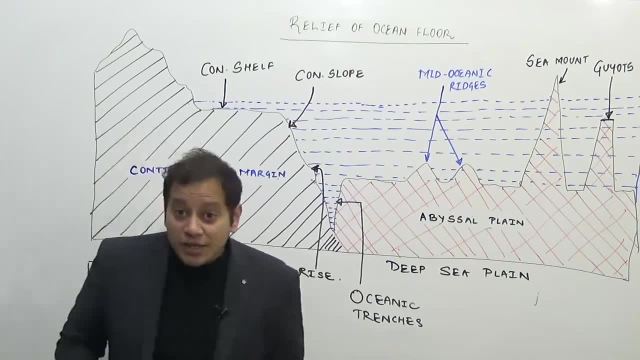 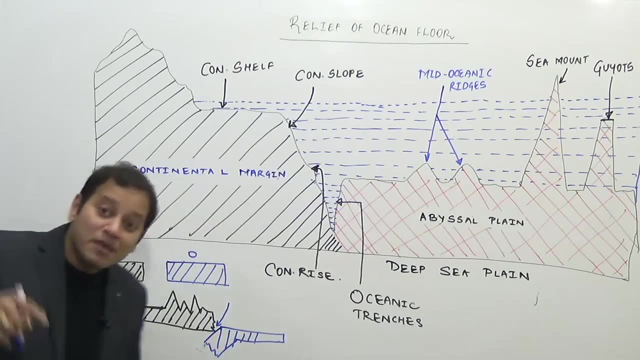 earth's surface are nothing but oceanic trenches. so what do they reflect? they reflect the subduction zone where the continental plate goes below the continental plate. so this is a boundary: oceanic plate has gone below the continental plate. if you remember the further lectures, these are the areas of a cold mountain. the oceanic plate melts. 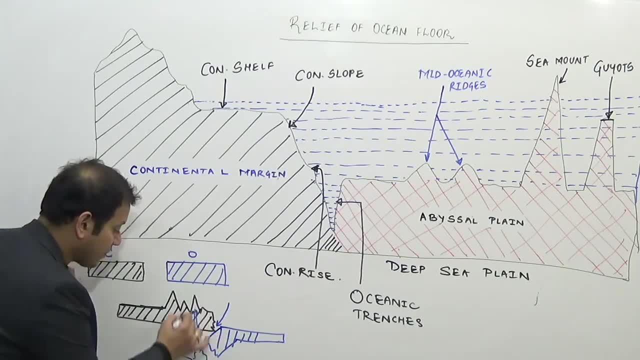 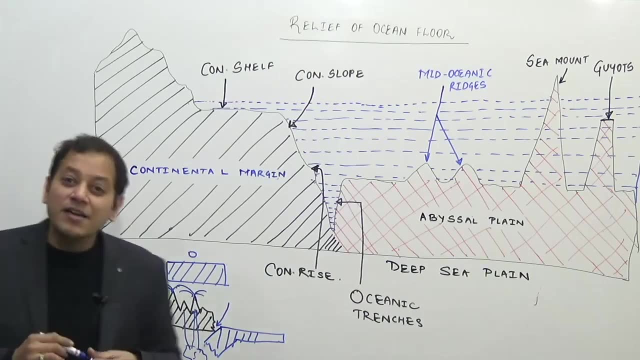 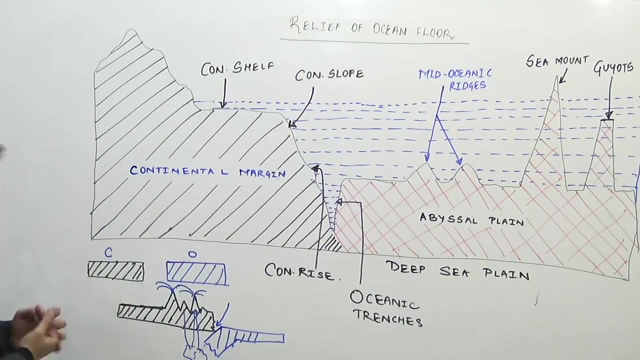 then it rises upwards the as magma and it blasts and it gives rise to the volcanoes of the world. so Pacific ring of fire again. if you remember those lecture, if you don't remember, please revise those lectures again. so if you know so it gives rise to most violent volcanic eruptions in this regions. so 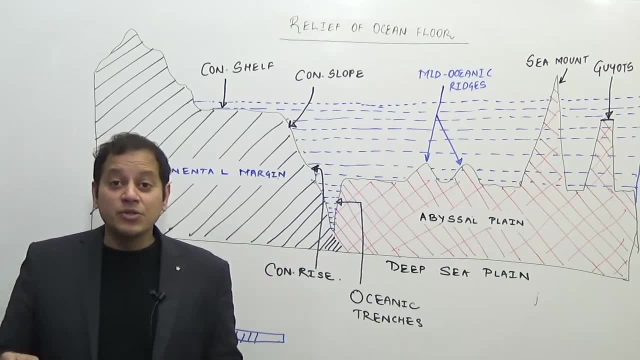 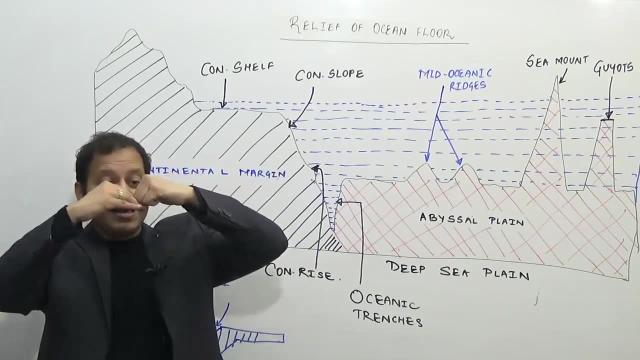 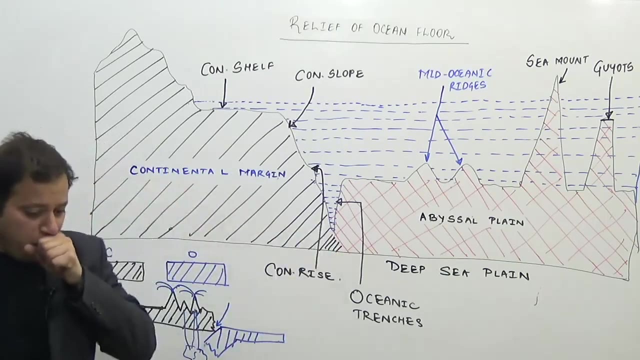 this is, oceanic trenches reflect the subduction zone or the area where the continental, where the oceanic plate goes below the continental plate. so this gap, what you can see, the gap between the two areas of my hand, is what is reflected on the earth's surface, what is here, here, we can see it. 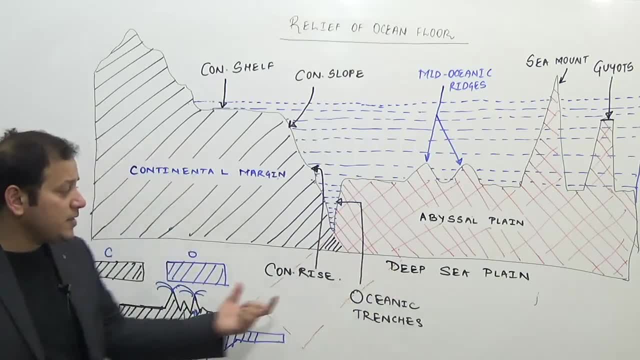 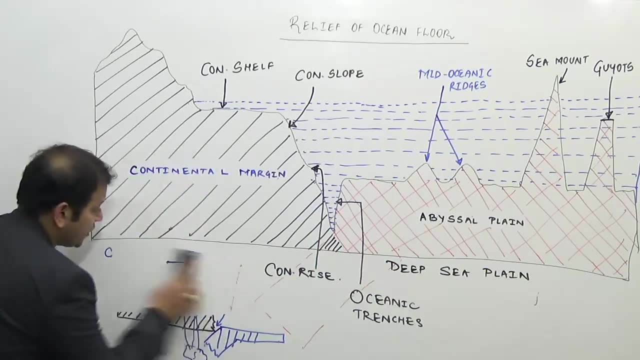 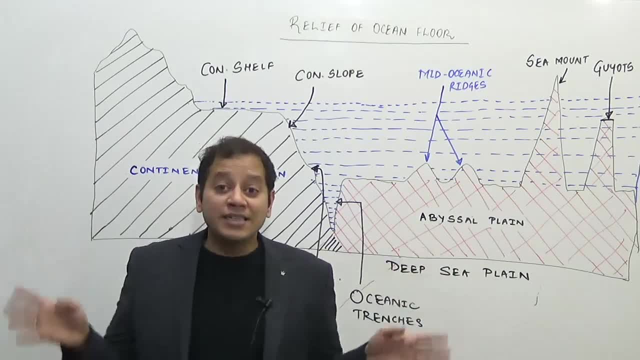 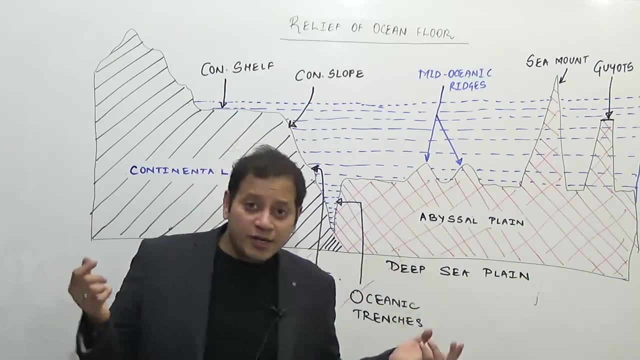 plates are not present everywhere. why this? oceanic trenches are not present everywhere? does India have a very, very deep trench nearby? yes or no, we will see here. India does not have a trench nearby. India has wide continental shelf. India has a deep or has a narrow continental shelf. 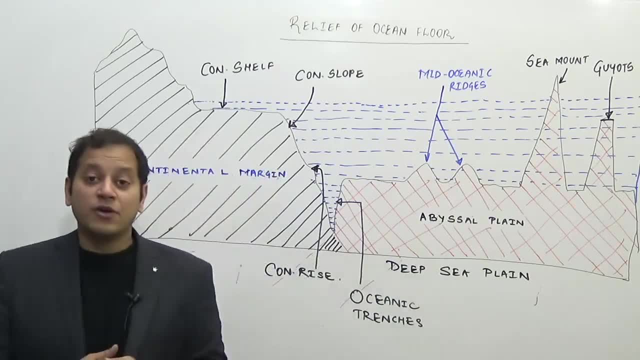 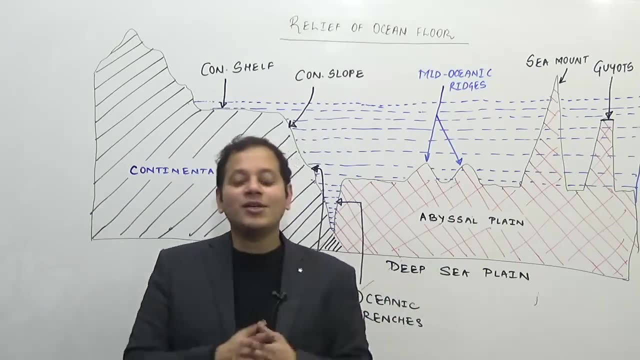 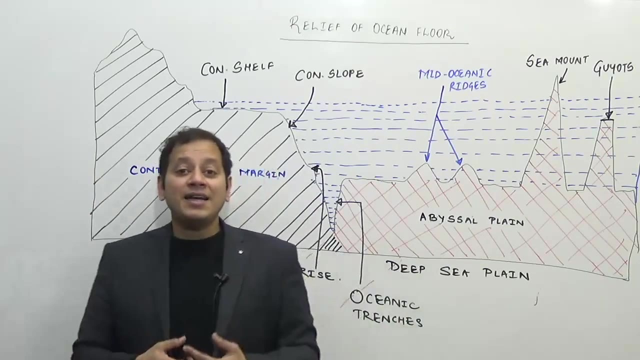 depending on the course, why there is a variation in the height of continental shelf, why goa is such a good place for tourism rather than the other things in goa. goa naturally also provides good sea tourism, good tourism industry. why is there some geography involved in it and why there is no continental shelf only? 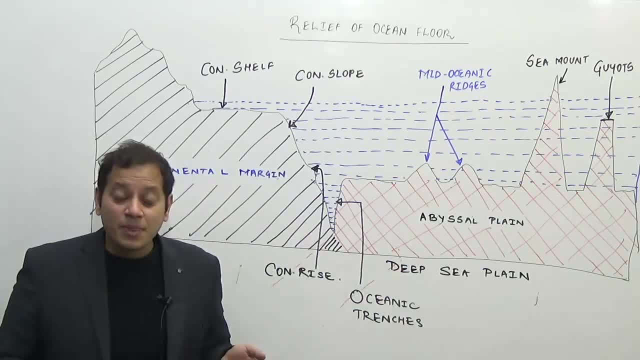 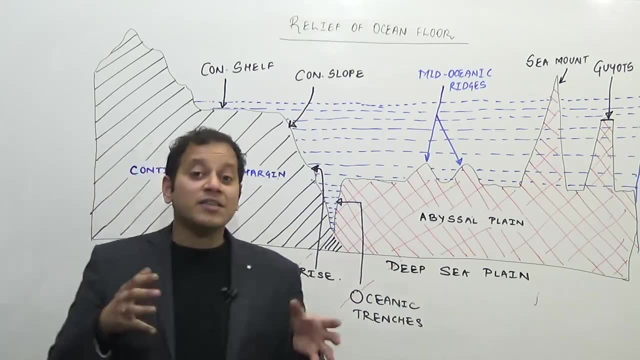 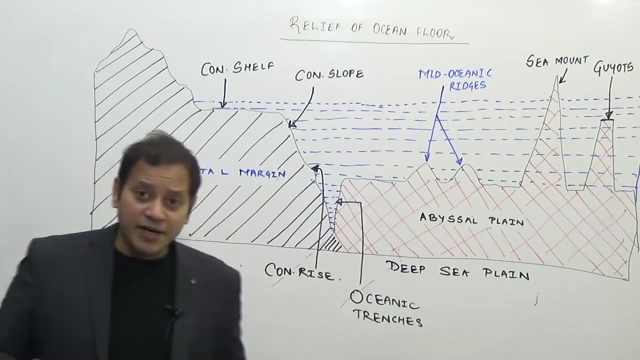 deep oceans, oceanic trenches near the oceanic trenches, near the south american coast, near the north american coast. so we will understand this while studying the different relief features in detail. but now you can remember that the continental margins are divided. the oceanic relief feature is divided into the continental 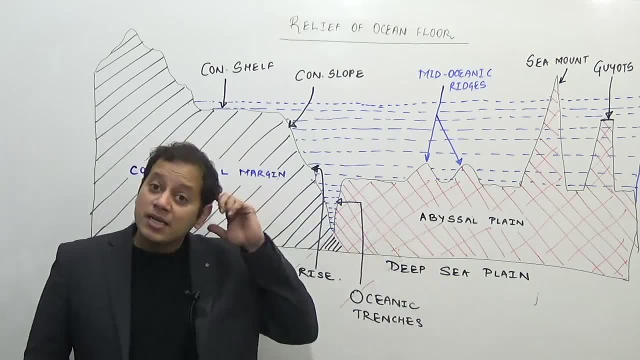 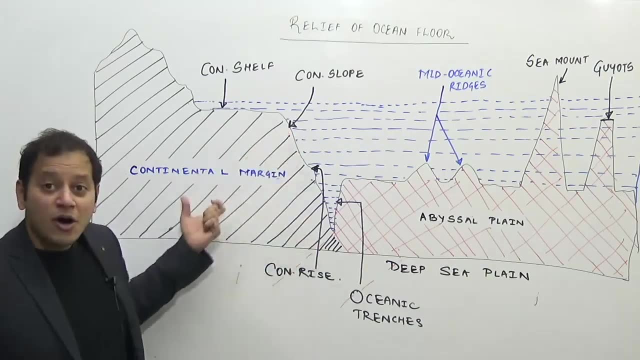 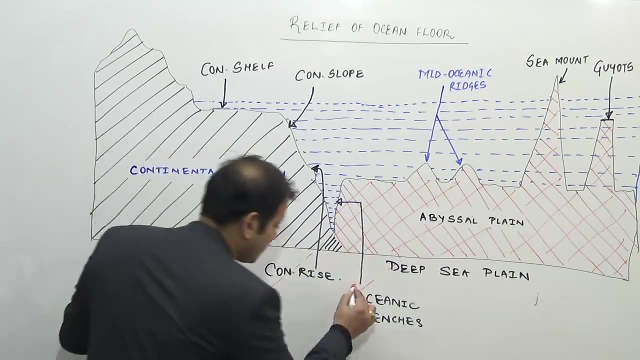 margins and into the deep sea plane, which is known as an abyssal plane. they are further divided into continental shelf, continental slope and continental rise. on the continental margin, while the deep sea plane, or the abyssal plane, is made up of oceanic trenches, mid oceanic. 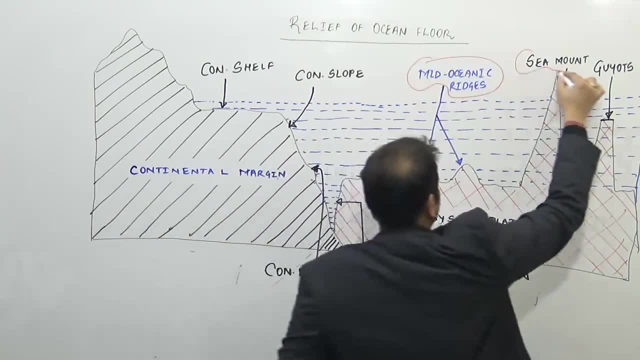 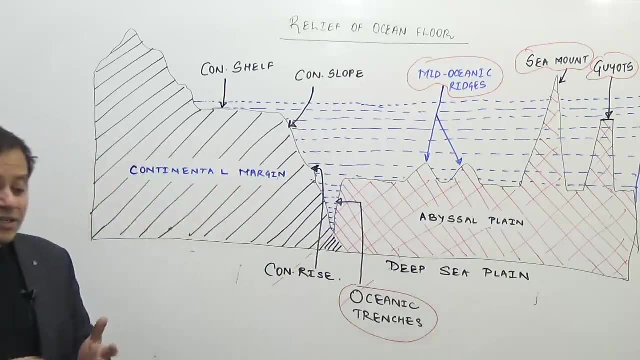 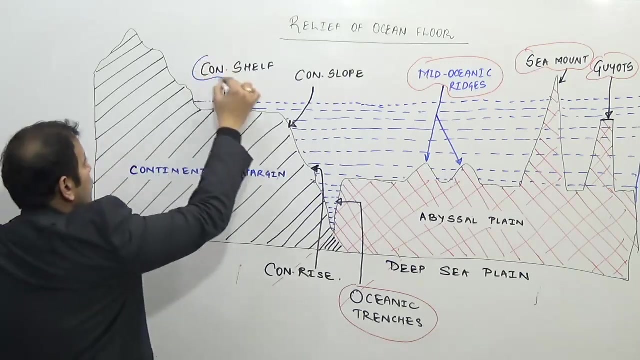 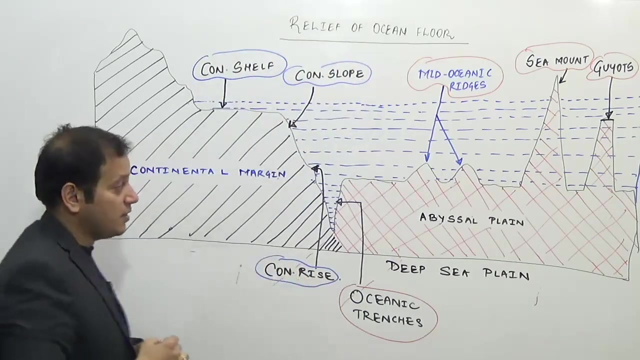 ridges, sea mounts and gears, and sea mounts and gears. so these are the four relief features of the of the oceanic margins, while the continental margins are made up of continental shelf and continental slope. why, while sometimes there is a continental rise, also obviously the dimensions of this that is continental. 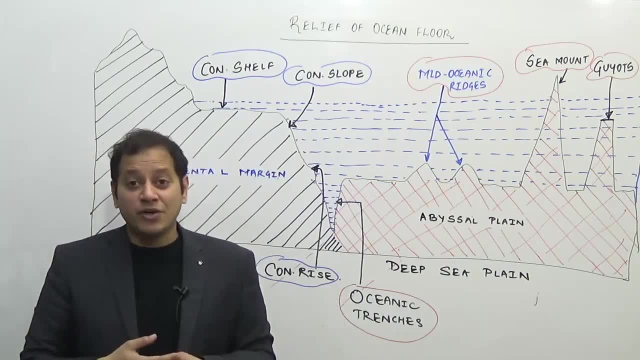 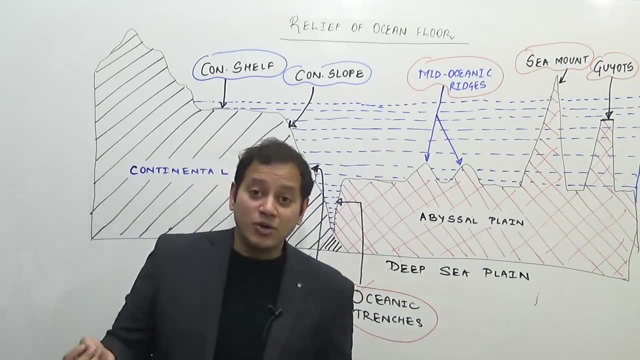 shelf the variation- and there will be variation- in the height of continental slope. the oceanic trenches may be present, may not be present. it all depends on the geomorphology or in the geology, or on the tectonics of the area. so this is how broadly a oceanic relief feature. 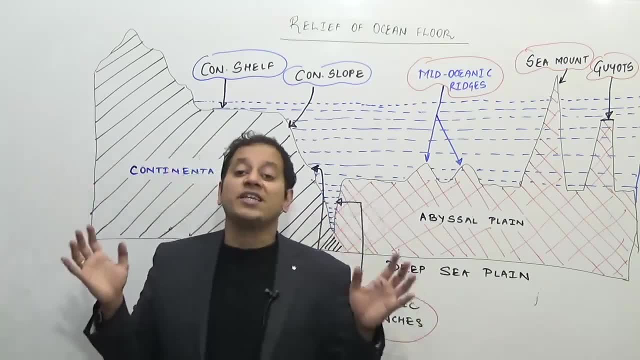 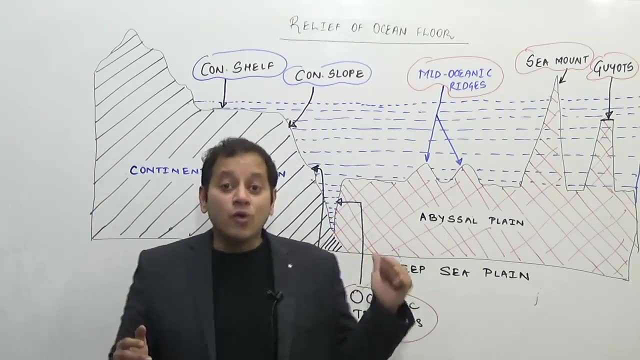 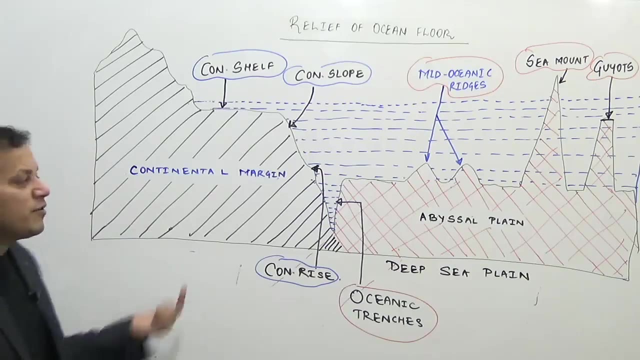 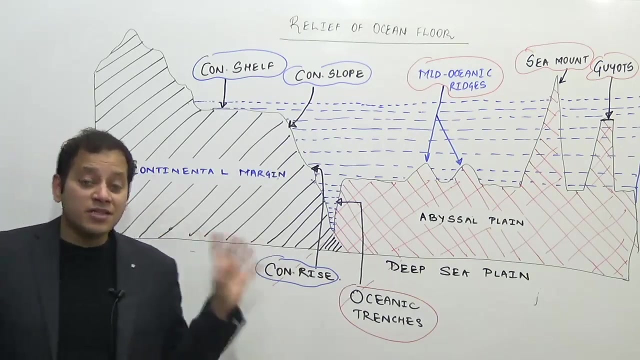 is divided into two, so two parts. this is known as an hypsographic curve or hypsogram. it is So metric curve. Now, before this, I hope that you have drawn the diagram. If you have not drawn the diagram, you are expected to draw this diagram in the examination. No need of shading that much, but obviously you have. you should draw this diagram. I hope that you understand what these features are. 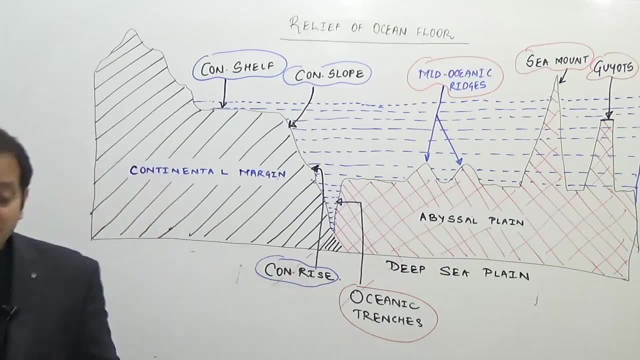 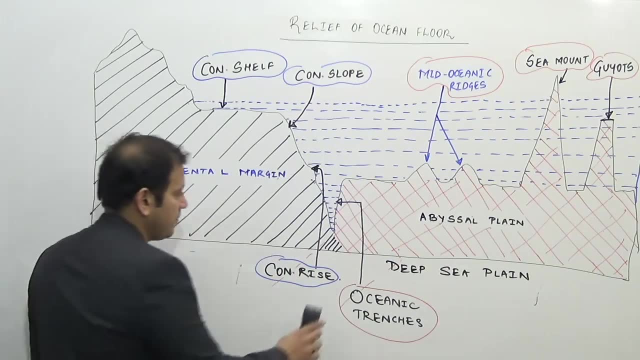 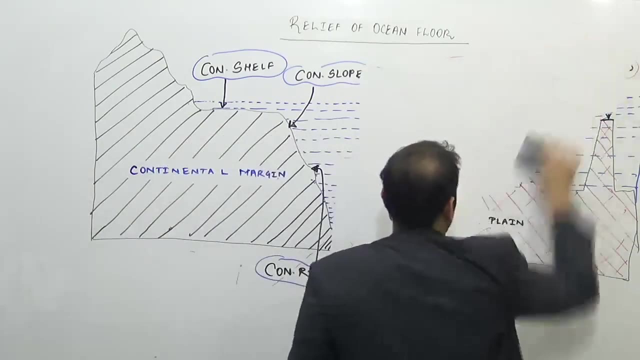 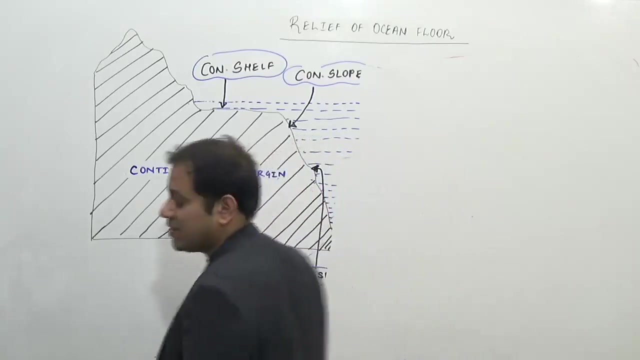 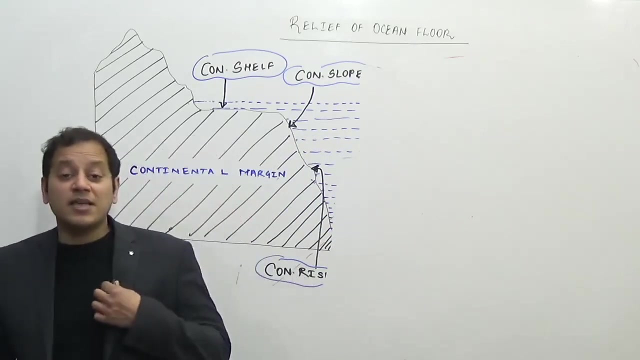 Now let us start with studying each and every feature in detail. I will rub this diagram now And I will keep only the three parts, that is, shelf, slope and rise. Now, what are the continents made up of? The continents? the continental margins are made up of continental shelf, continental slope and continental rise. 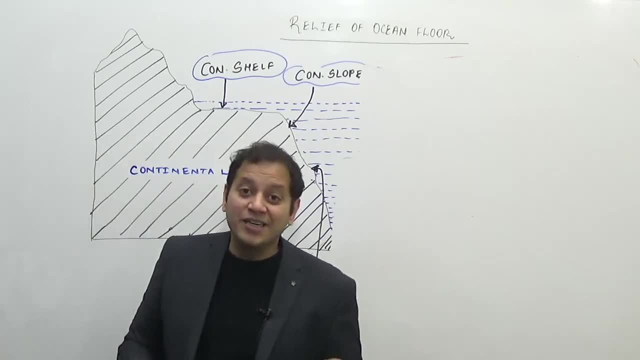 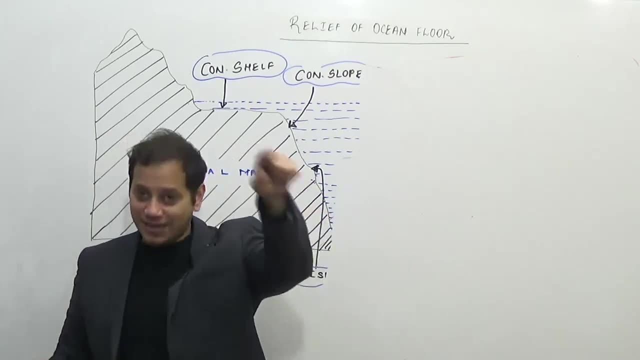 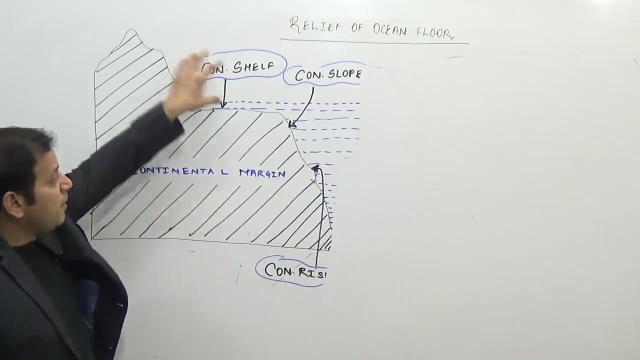 The continental margin is a part of an continent which is below the ocean and therefore the dominant material is granite or basalt. It is granite here. The most dominant material is granite in this part. Now it is further divided into shelf slope and rise. So let us study what. 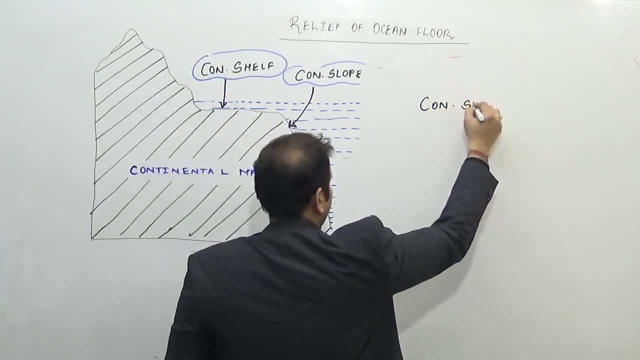 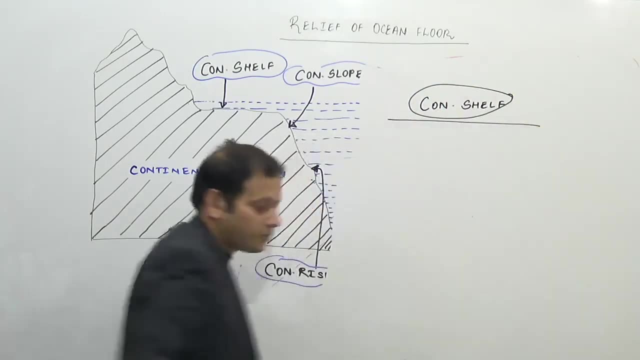 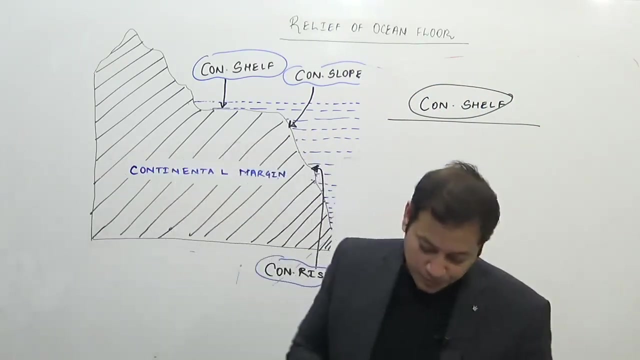 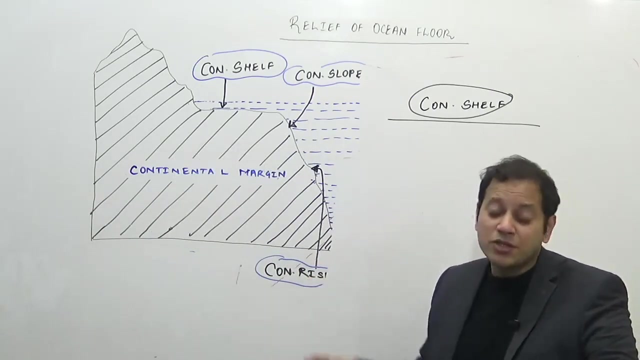 is this continental shelf? What is this continental shelf? What is this continental shelf is a gently sloping area which is near the edge of a continent, which is below the ocean, a gently sloping area having a very gentle slope seawards and seawards. So this is a continental shelf, So this is a continental shelf, So this is a. 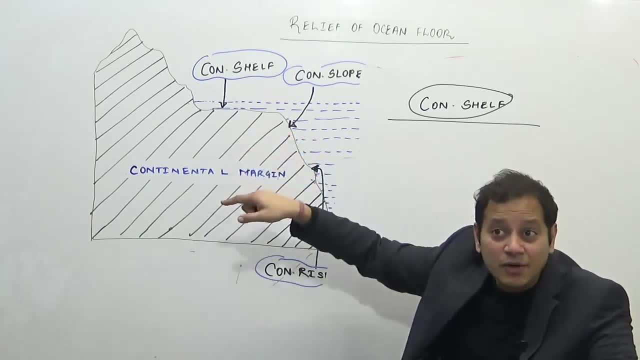 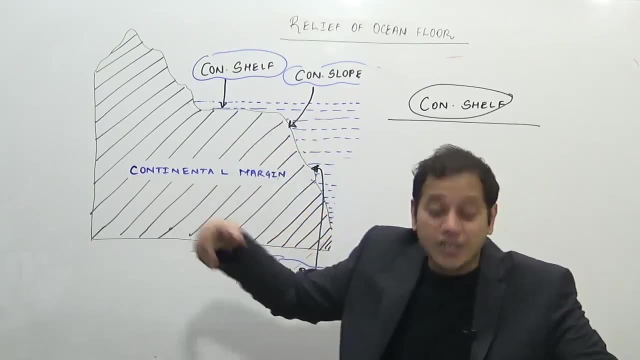 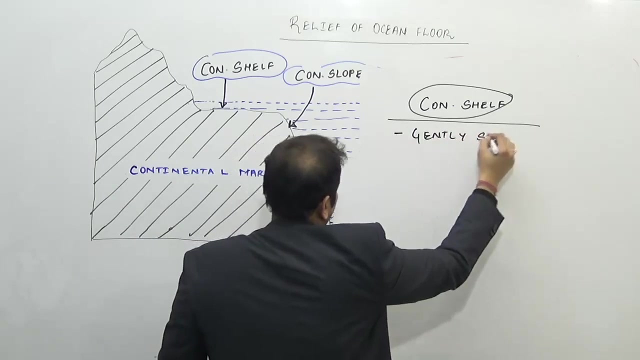 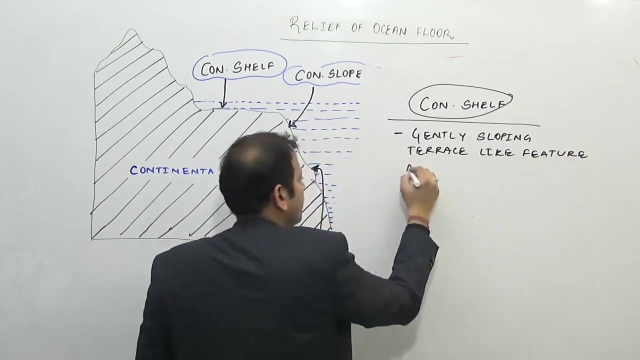 continental shelf. and what is the depth? Is the depth greater or narrower or shallower? Not narrower, obviously shallower. Having a shallow depth is known as a continental shelf. So a terrace like flat, gently sloping feature. terrace like feature. Now the slope is at the edge of a continent. 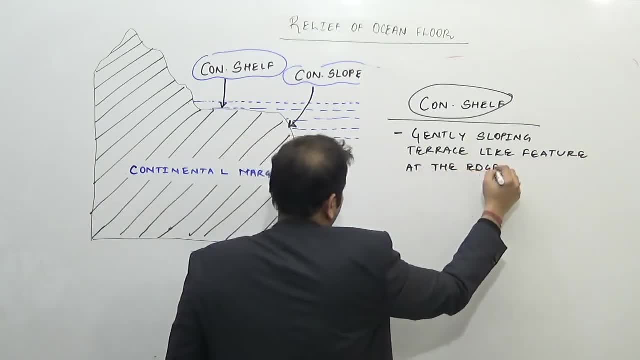 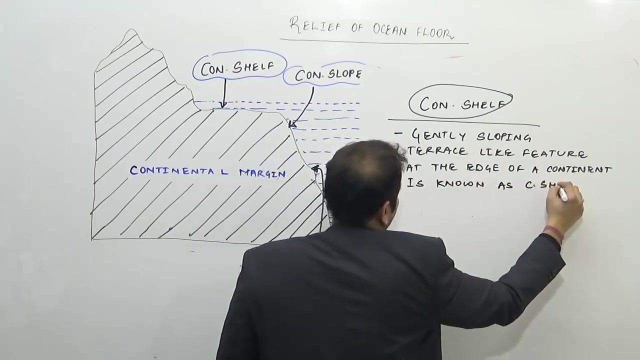 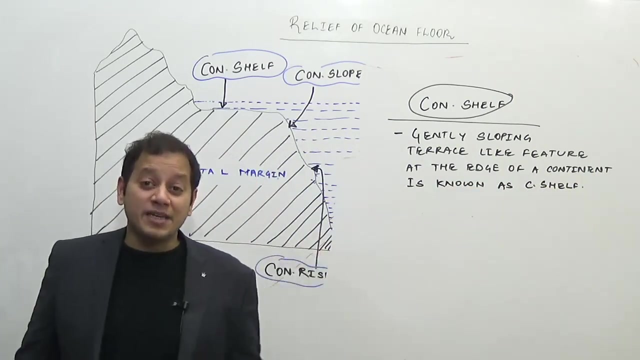 The slope is at the edge of the continent. Continent is known as continental shelf Is known as continental shelf. What is the slope? The slope is extremely gentle, of one to two degrees slope. Now the continental self is known as a continental shelf. 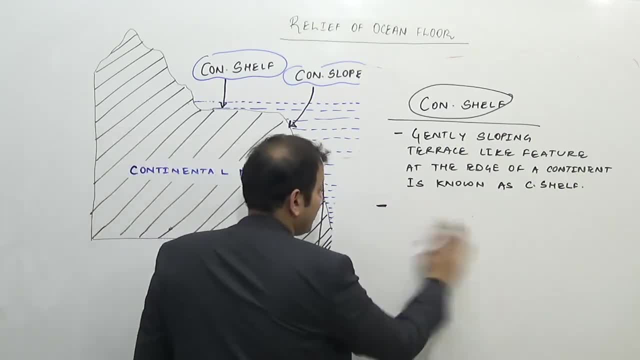 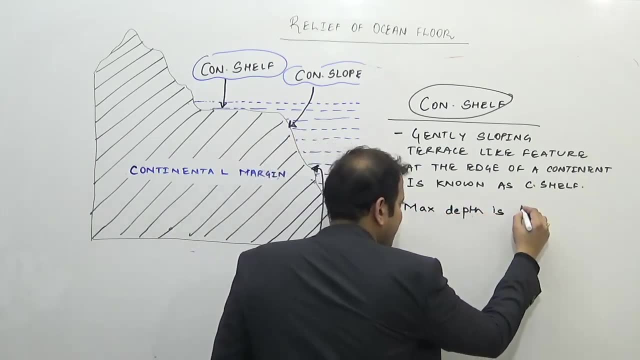 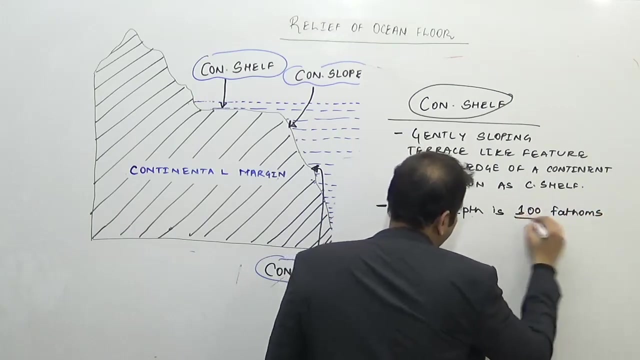 continental shelf. i Dy describes a slope of one degree slopes. now the Boulevard slope of a continent shelf is of a shallow depth. the maximum depth is is hundred fathoms, hundred fathoms. the maximum depth is around hundred fathom when one fathom is equal. 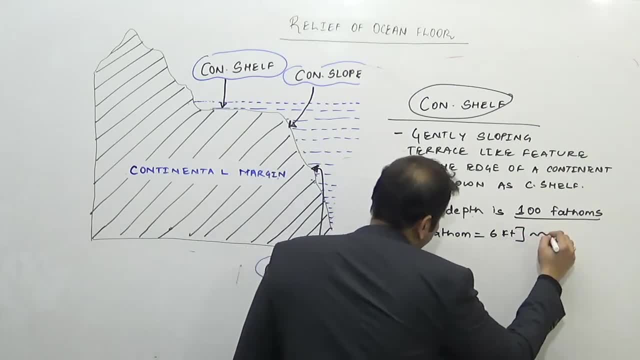 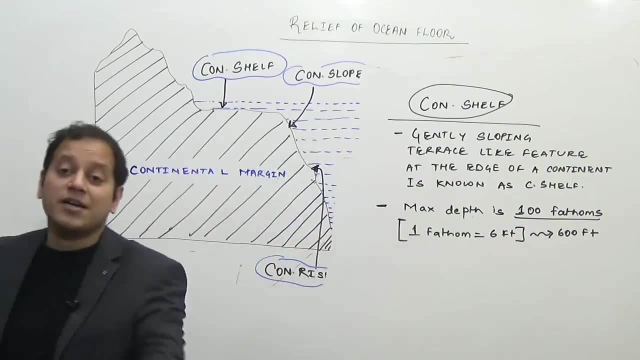 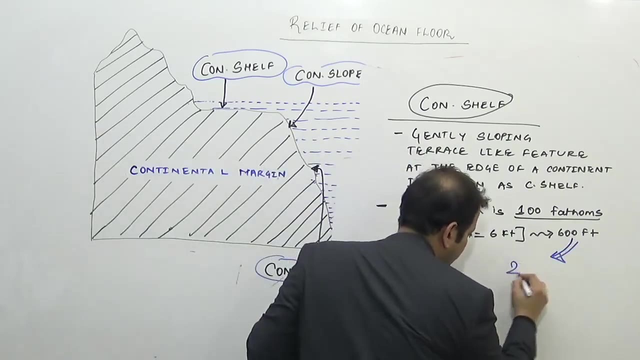 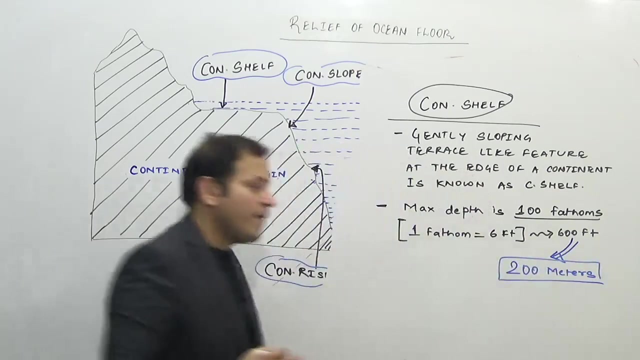 to six feet. that means maximum depth will be around 600 feet. the maximum depth is around 100, 100 fathoms or 600 feet, or we can say it will be around 200 metres. it will be around 200 metres. it will be around 200 meters, so it is having a maximum depth of around 200. 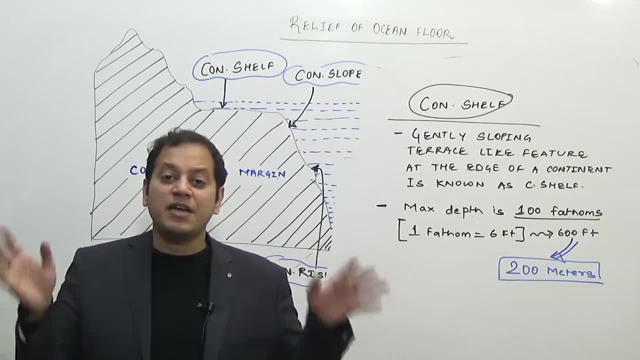 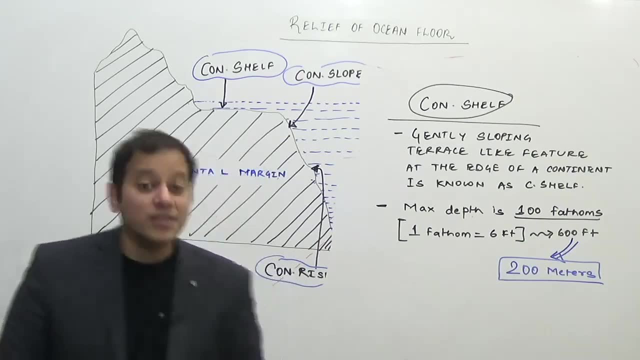 metres. a flat, generally sloped, sloping, terrace-like feature having a maximum depth of around 200 meters and a slope of around 1 to 2 degrees is known as a continental shelf. Now the next is if, again your geomorphology class, again your climatology class. See these parts which we will be doing from this lecture. 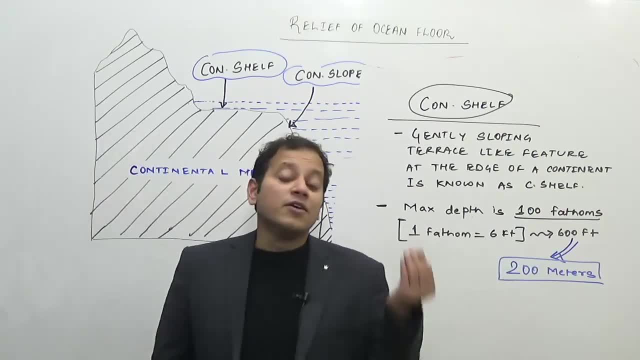 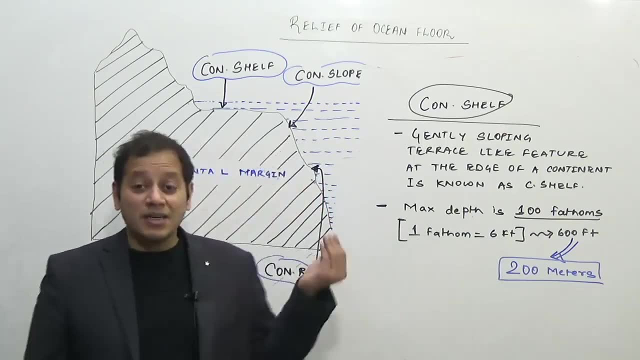 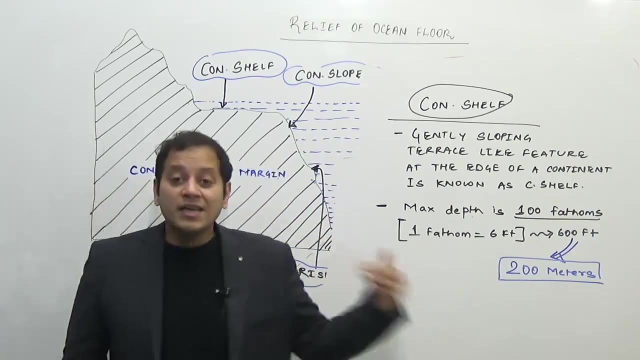 series onwards. they will be very simple and very fast. Unfortunately, I was not well for so many days and therefore the lecture series was, you can say, postponed, but now they will be very much regular. I am extremely sorry for the inconvenience caused to you, but now here we will be regular in. 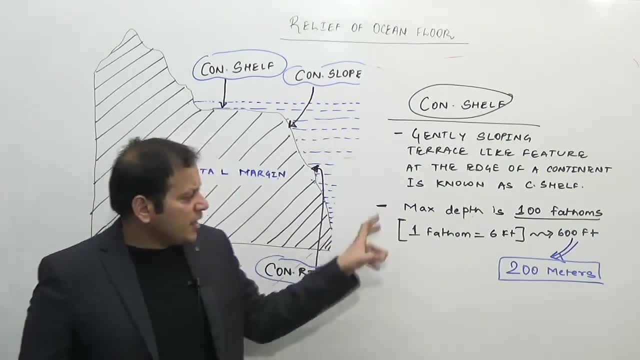 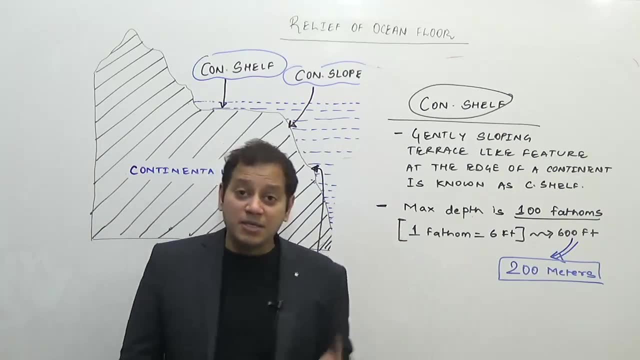 this studies now of the oceanography. Now here, the maximum depth is 100 fathoms, or we can say the maximum depth is around 600 feet, because 1 fathom is equal to 6 feet, or the maximum depth is 200 meters. Now, if you remember your climatology lecture, the sunlight can penetrate maximum up to 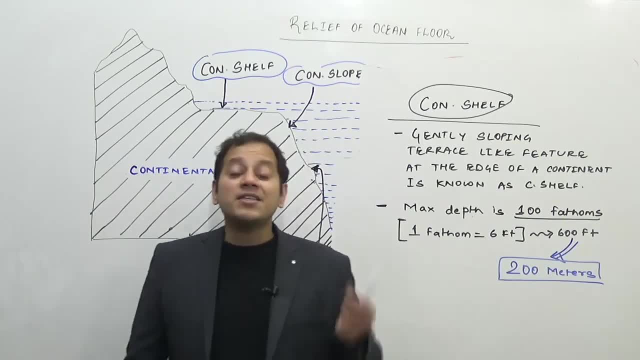 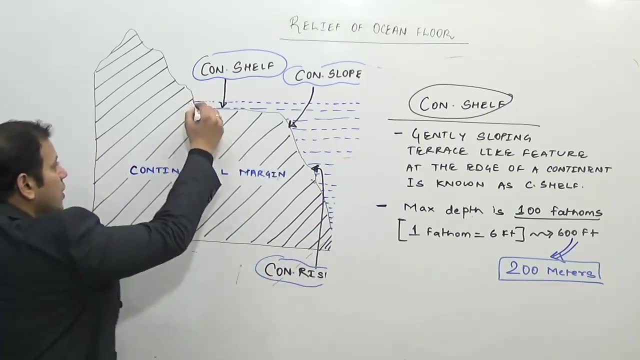 200 meters Inside the ocean. this is known as an photic zone. Therefore, the sunlight can penetrate here in the continental shelf, giving rise to what are known as plants or plantains in the continental shelf region. So there are numerous corals, numerous plantains. 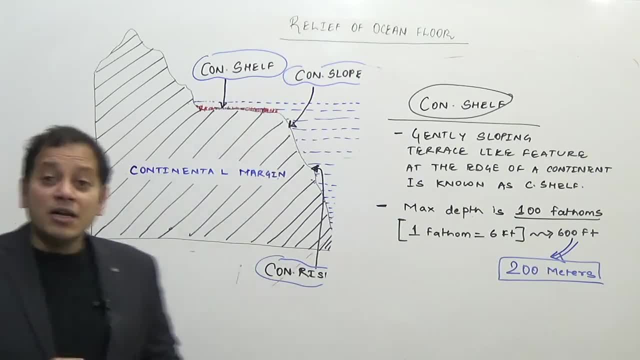 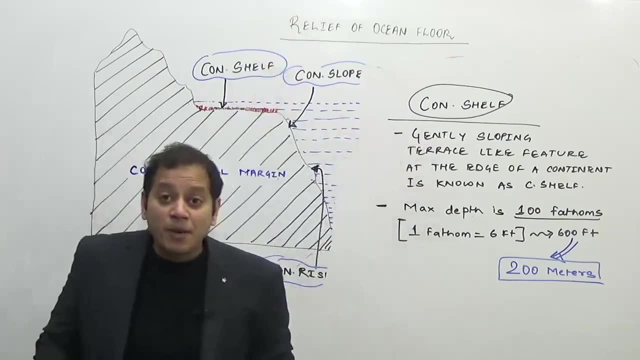 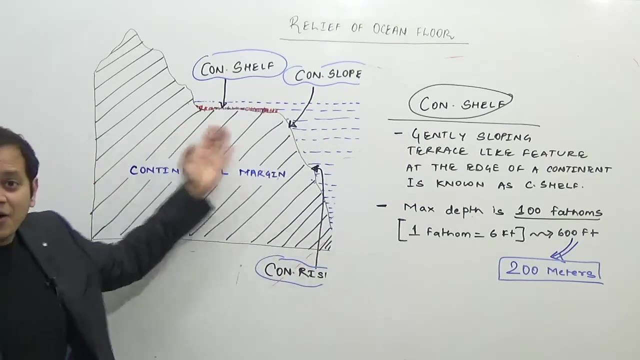 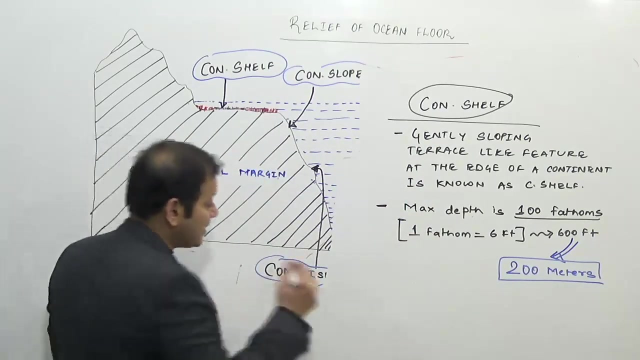 numerous plants in this continental shelf region. Now, what will be the deposits on the continental shelf? Will it be deposits from the land, or will the deposits will be from the ocean? The deposits on the continental shelf will be from land or from the deep sea? Obviously, the deposits will be from the land surface. So you remember, these are covered by pterygineous deposits. 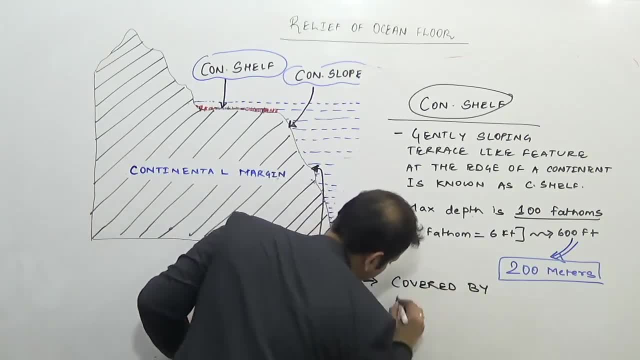 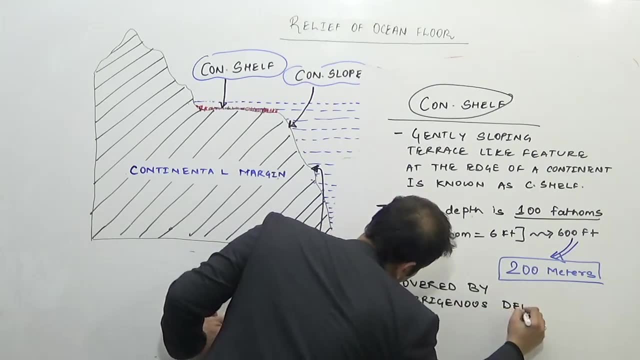 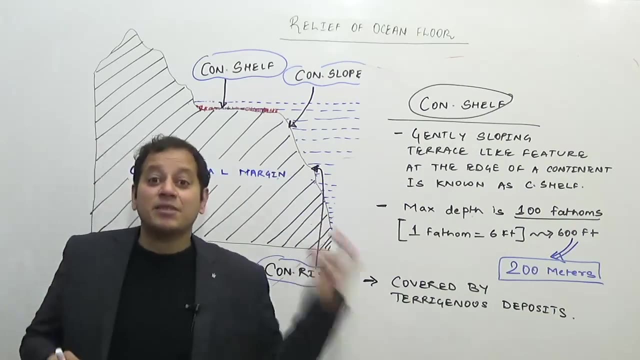 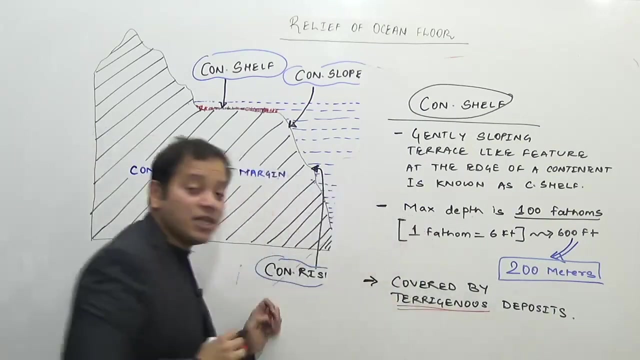 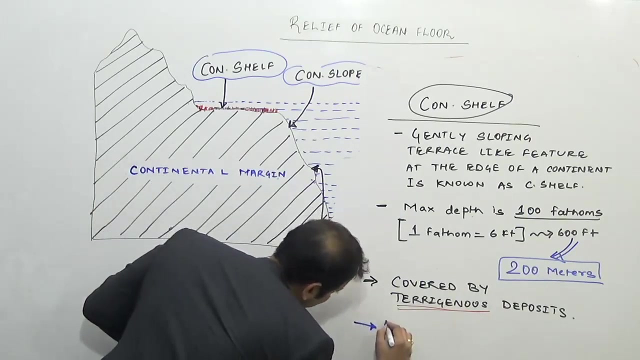 These are covered by pterygineous deposits. These are covered by pterygineous deposits. What do you mean by pterygineous deposits? Ptery means territory, land, and genus means origin. So this area is covered by deposits which are originated on the land surface. Therefore, pterygineous deposit, because it lies in the photic zone, because it lies because the sun rays can penetrate. 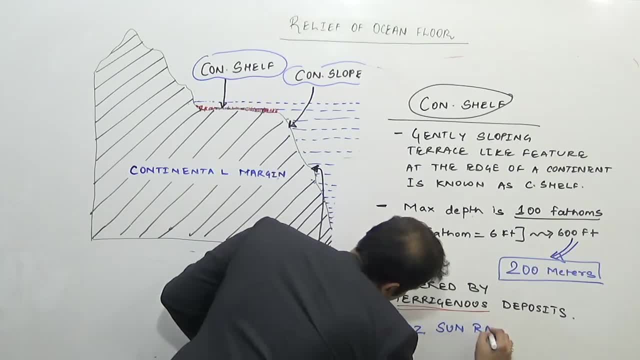 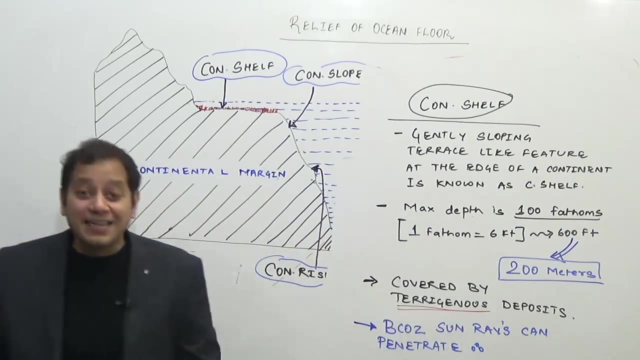 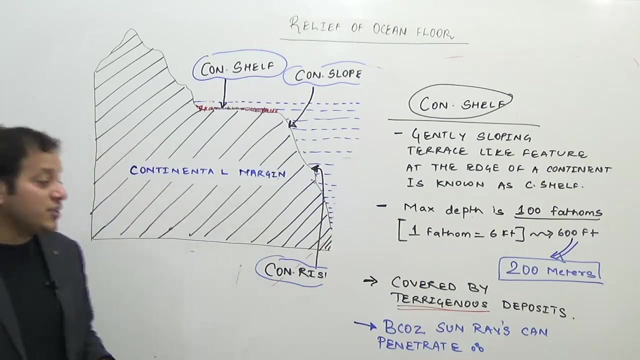 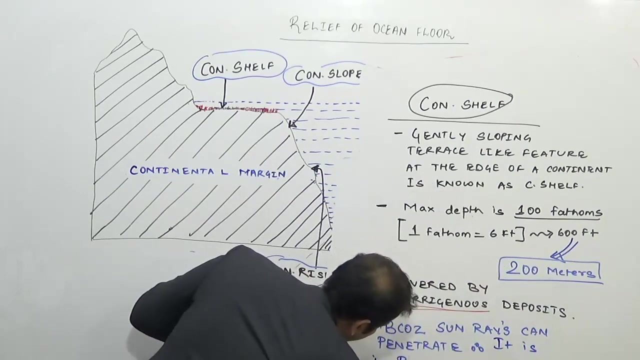 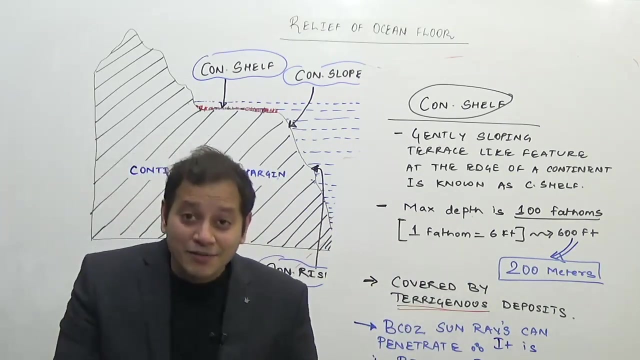 Sun rays can penetrate. Therefore, there are large number of plantains, there are large number of sediments, there are large number of marine life in the continental shelf area. Therefore, it is rich in biome. It is rich in biodiversity. Now the blue colored point. if it is rich in biodiversity, what do we get from the sea? We get food from the sea. we get energy from the sea. we get numerous of relief features. we get numerous of economic resources from the sea. 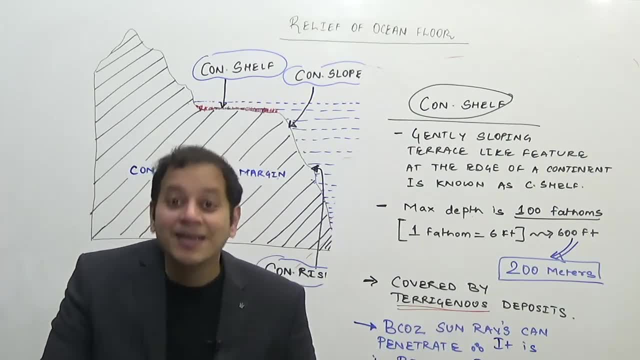 Now the blue colored point: if it is rich in biodiversity. what do we get from the sea? We get food from the sea. we get energy from the sea. we get numerous of relief features. we get numerous of economic resources from the sea. 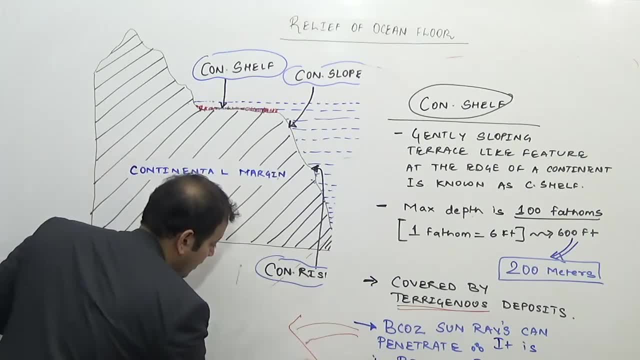 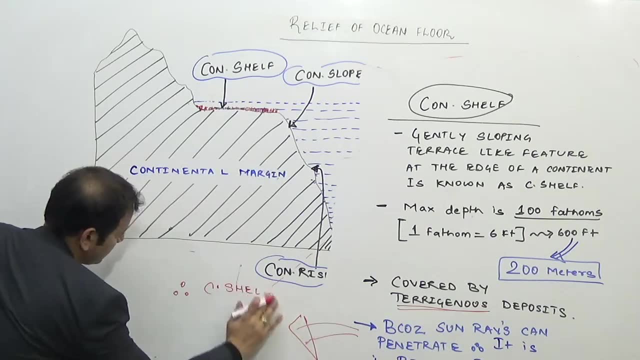 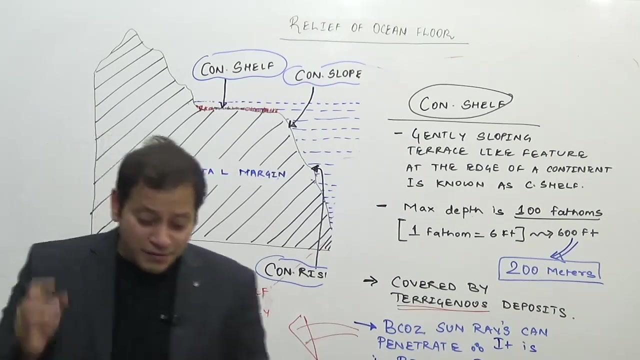 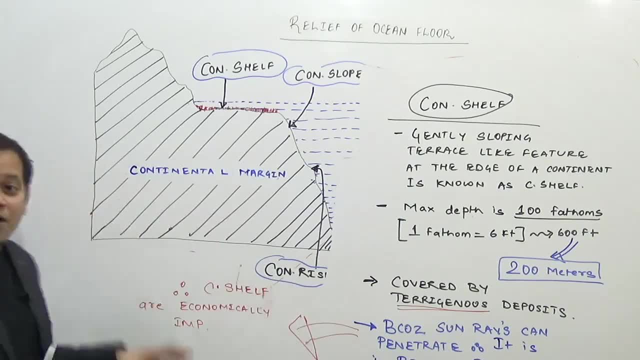 of an continental shelf. the depth of a continental shelf or the width of a continental shelf will keep on varying and therefore, because of there will be variation in the continental shelf, there will be variations in the continental shelf, in continental shelf, and this is what we are going. 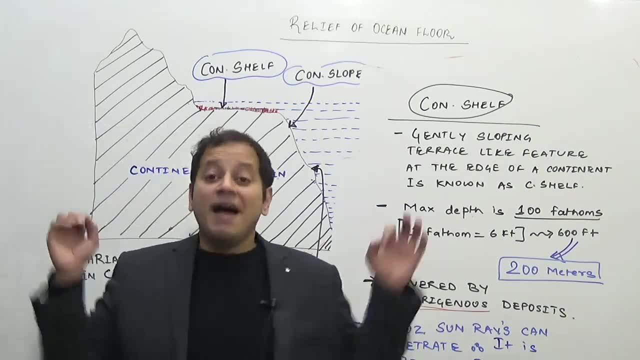 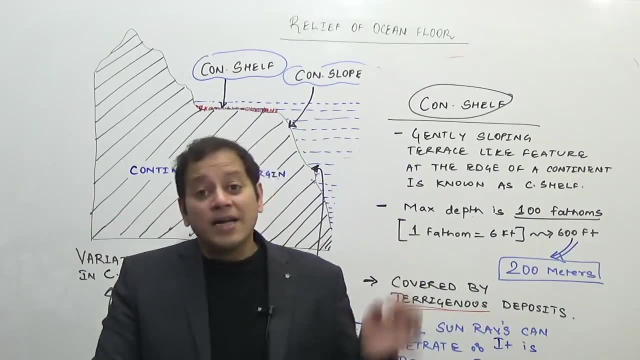 to study the variations in the continental shelf at the end of the this variation. studying the variation in the continental shelf, you will be able to understand why there is more continental shelf in some parts of the world while less, why some areas are rich in petroleum deposits, some 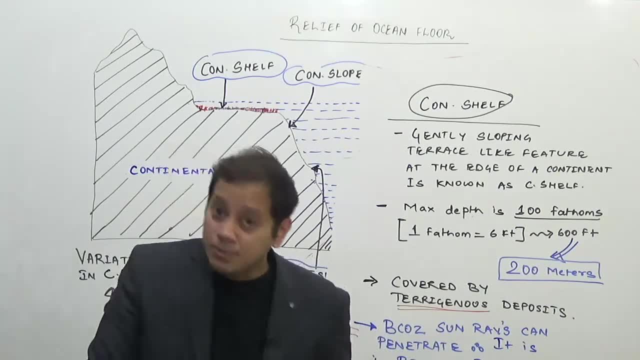 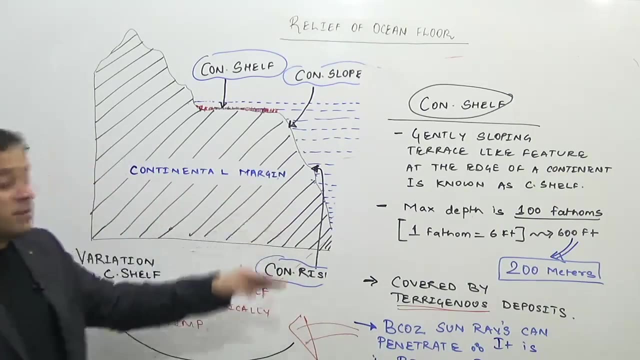 areas are rich in fishing deposits, while some areas are poor. and also you will be able why gulf of kutch region is is famous for tidal energy. okay, so what is this continental shelf? it is a gently sloping terrace, like feature at the edge of a continent. maximum depth of thousand of 600 feet, that is, 100 fathoms. 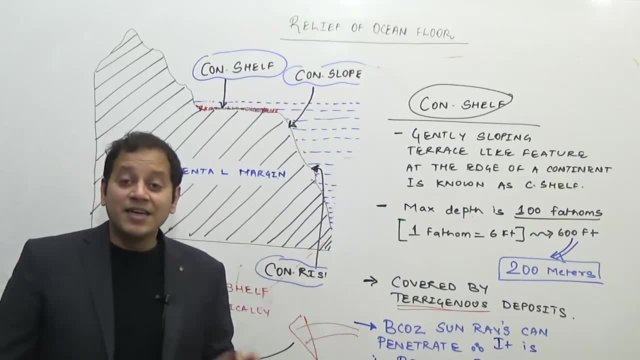 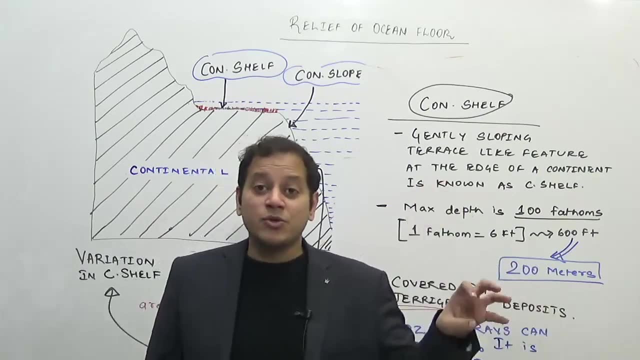 covered by terriginous deposits because the light can- sunlight can easily penetrate. therefore the plants known as phytoplanktons on which the fishes depend, which are the major ohs, which are the lowest in the biome of the oceanic biome, which are the manufacturers of food. 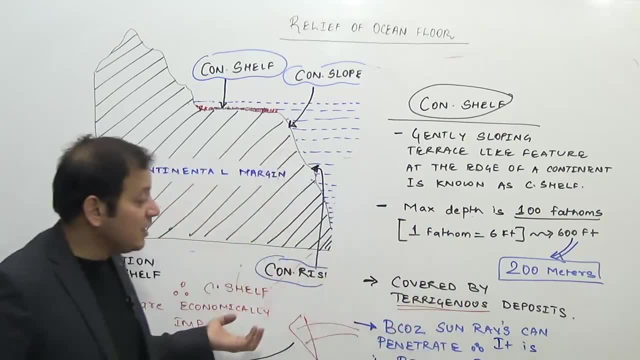 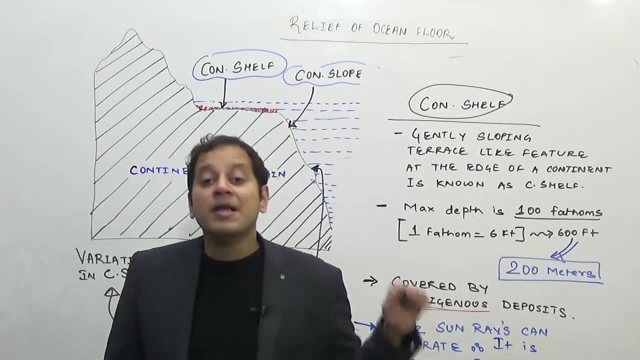 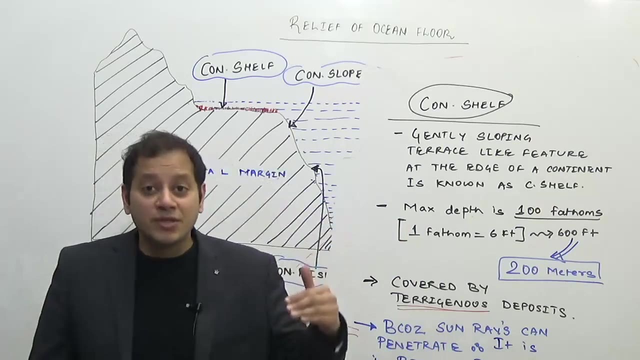 through photosynthesis in the oceanic biome can easily thrive. so these are the producers of verschiedenen biome food chain. if you know, environmental ecology, far the food chain desire lie at the bottom of a fortune and therefore anything which lies on the bottom of the food chain are producers and they produce food on which we, because we cannot produce our own food, we cannot. 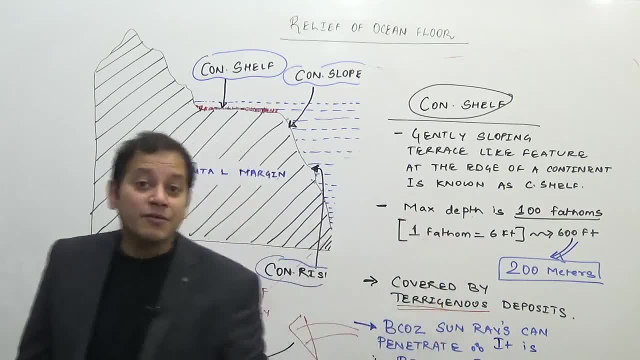 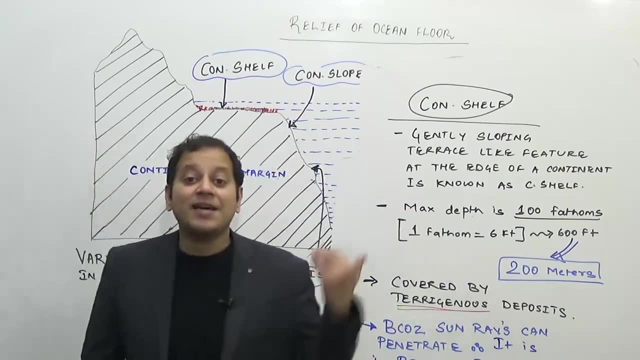 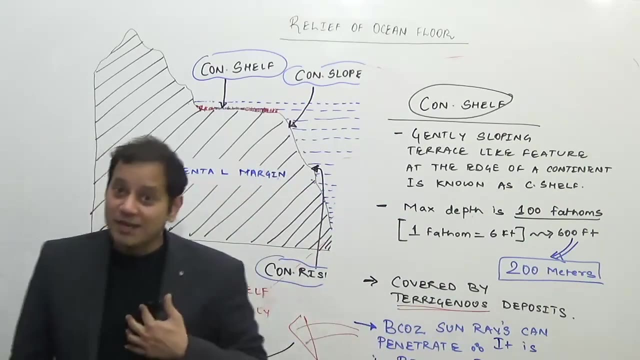 we are consumers. we eat plants by. we cannot use the energy from the photosynthesis, so we eat this. plants, even in the marine biome, fishes and other marine organisms depend on this phytoplankton. so this are rich in biodiversity. when they are rich in biodiversity, the economic man has used. 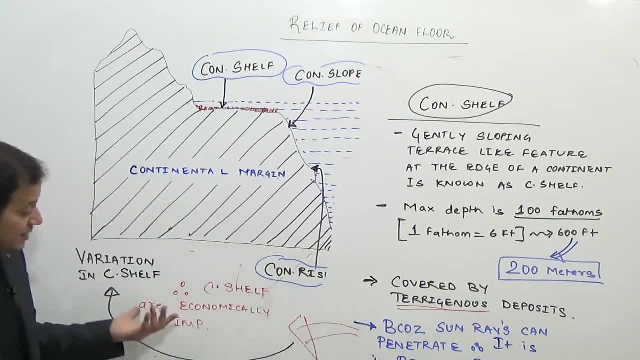 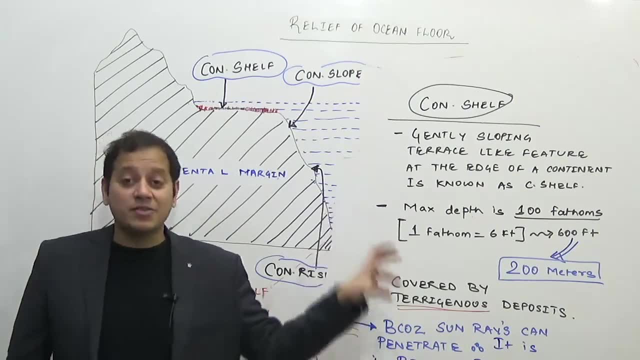 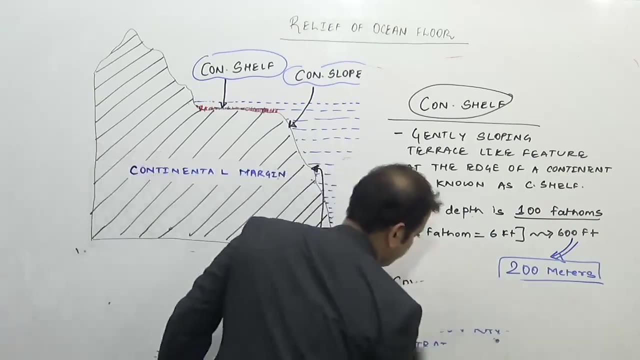 these animals for their own consumption and therefore these are the. these are of economic importance, but remember, there is a variation in the shape and the size of a continental shelf, which we will do before the. before that we will study what is the continental slope. before that we will study the continental slope. 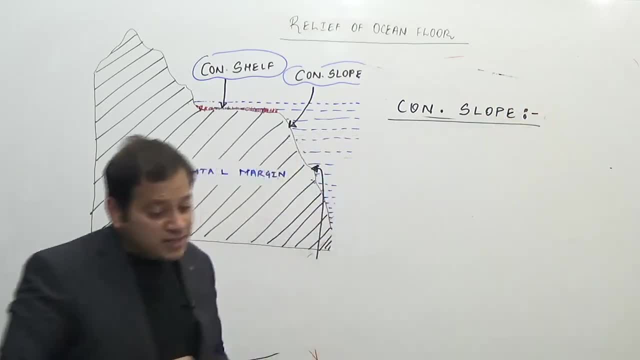 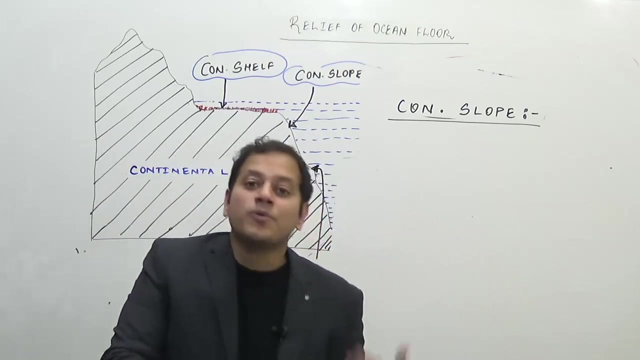 now, what is this continental slope as a steep seaward slope? now, obviously it is a steep seaward slope having having a steep slope, a seaward region at the end of a continental shelf having a steep slope. so we can write it as a steep seaward slope of two to five degrees, having a greater depth of. 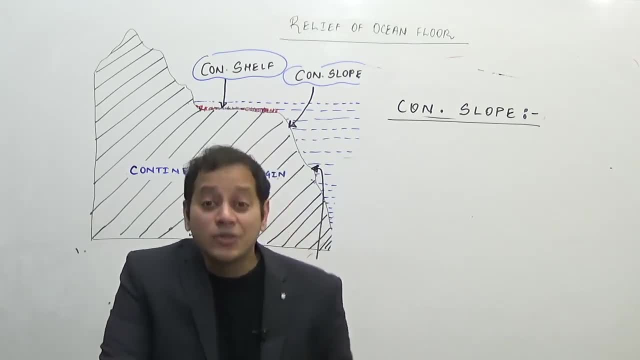 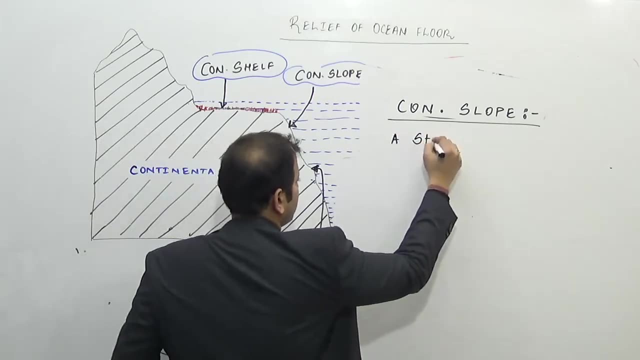 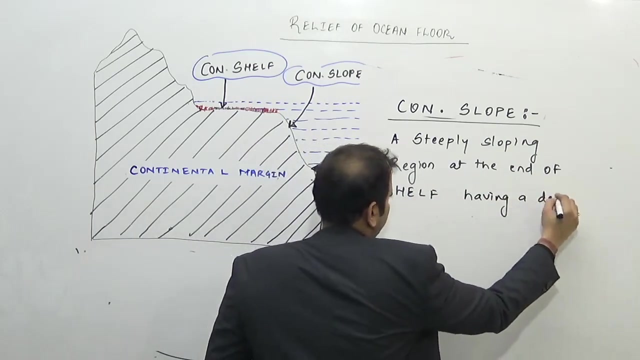 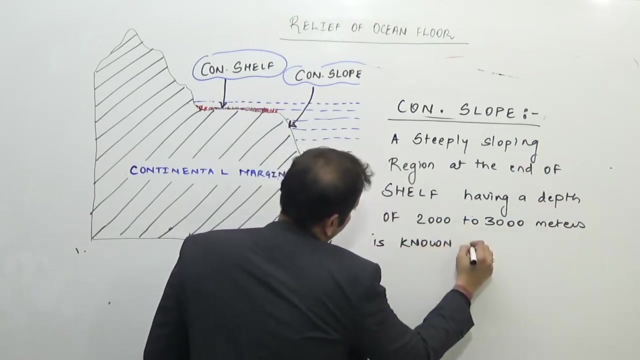 around three thousand two thousand to three thousand meters is known as an continental shelf, so a steeply sloping at the end of shelf. at the end of shelf having a depth of of two thousand to two or three thousand meters is known as is known as continental slope. 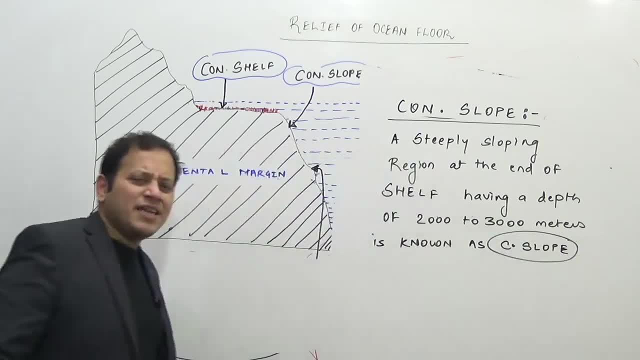 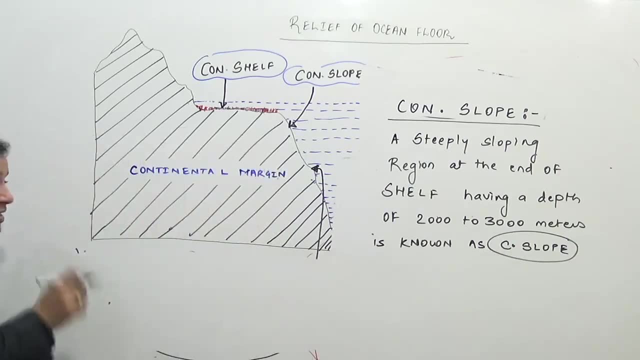 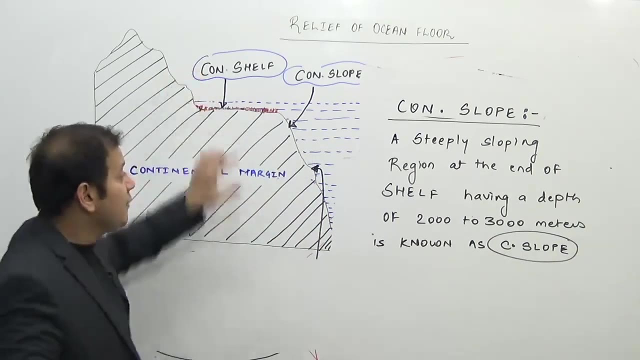 so it is a steeply sloping region. obviously it is not rich in any deposits because the sunrise cannot easily penetrate also. thus, also because it is a steeply sloping region, whatever the deposits are are derived from the land. yeah, if they come on the continental slope region, they do not stay here, but they come downwards. 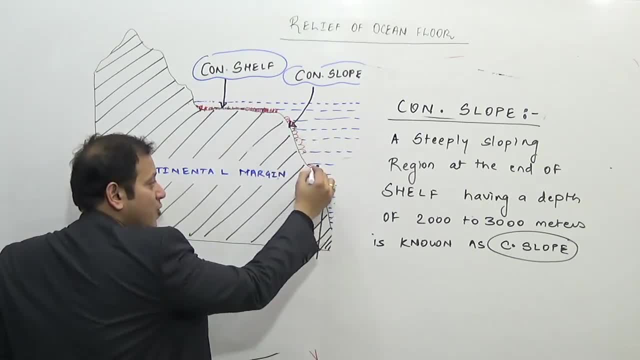 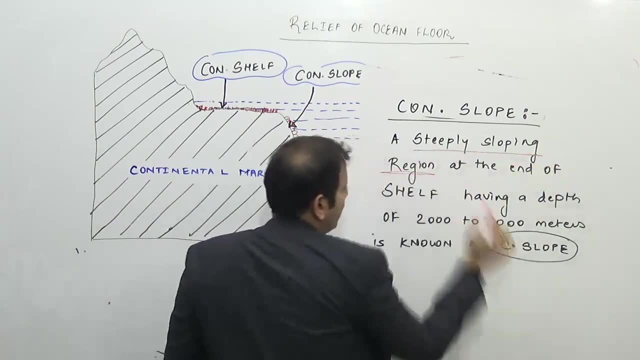 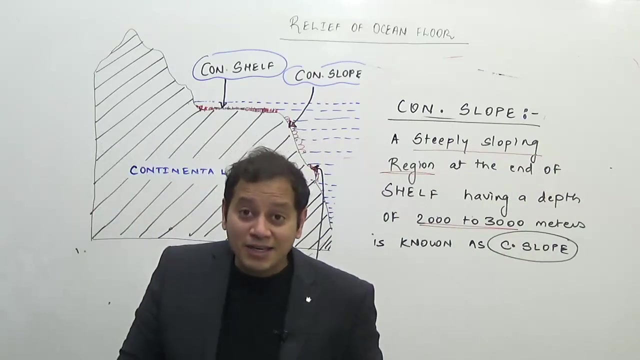 they move downwards because of the steep slope and they get accumulated in this region. so what you have to remember, it is a steeply sloping region. at the end of a shelf having a larger depth now, because of the steepness of the slope, the deposits do not stay on the continental slope. 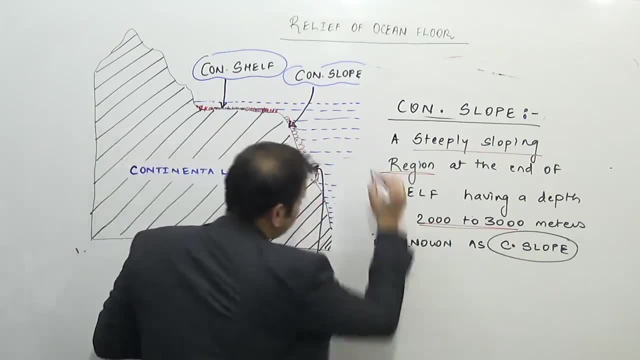 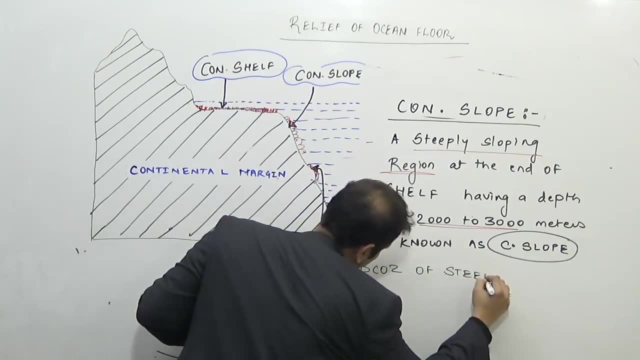 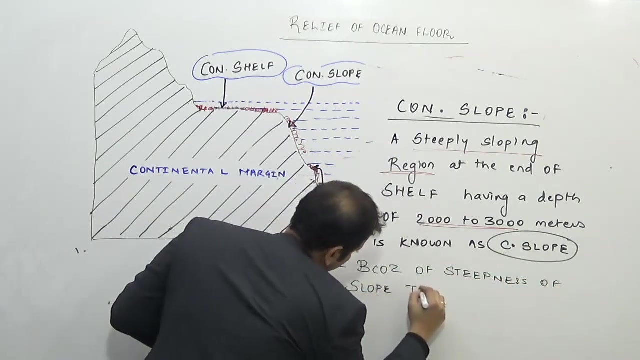 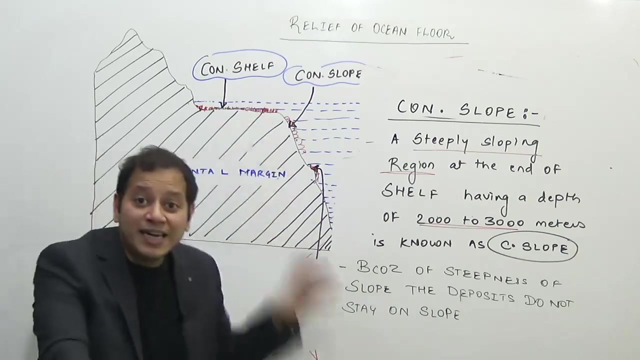 and because of the steepness, because of the steepness of the slope, the deposits do not stay on slope. if they are not staying on the slope, what will be the deposits doing? the deposits will roll down and get accumulated at the end of a slope because there the steepness ends, so they will get. 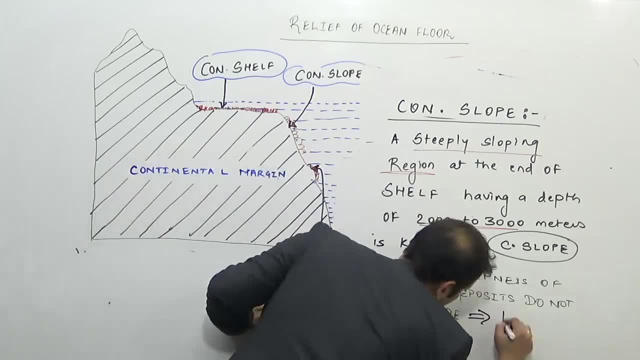 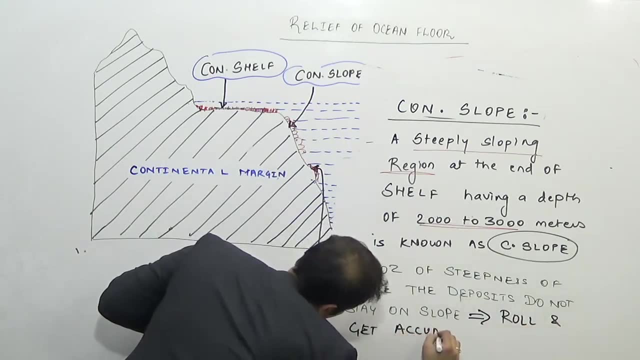 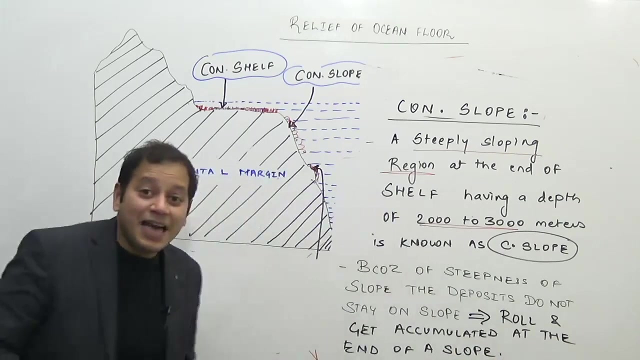 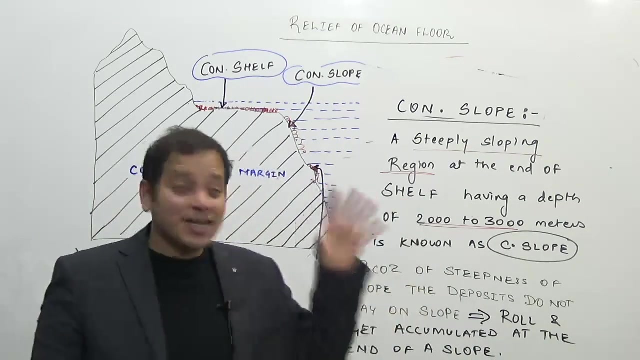 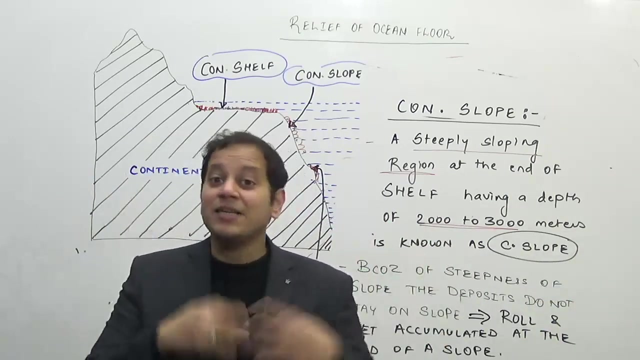 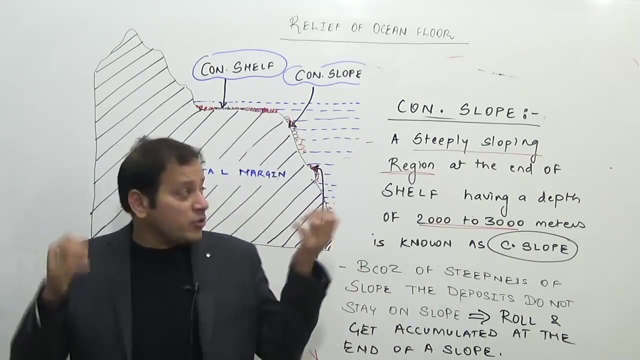 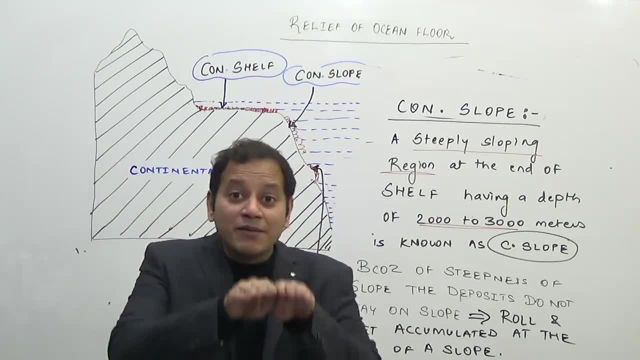 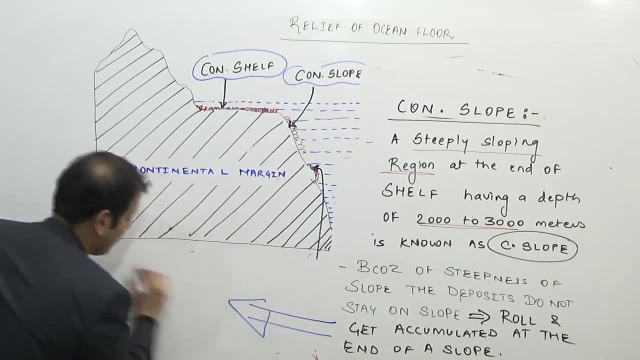 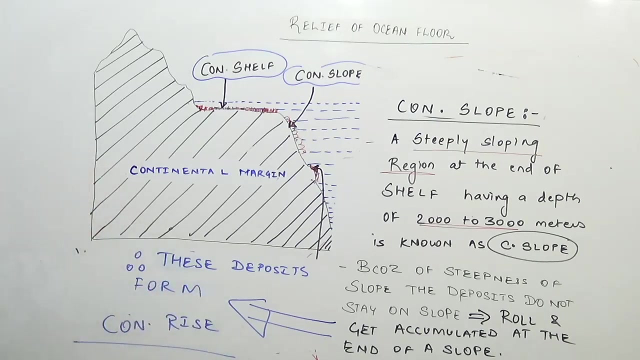 a slope and therefore, at the end of a continental slope there will be slightly rising area, what we call as an continental rise. So therefore they give rise, these deposits give rise to continental rise, or these deposits form continental rise, These deposits which get accumulated form continental rise. 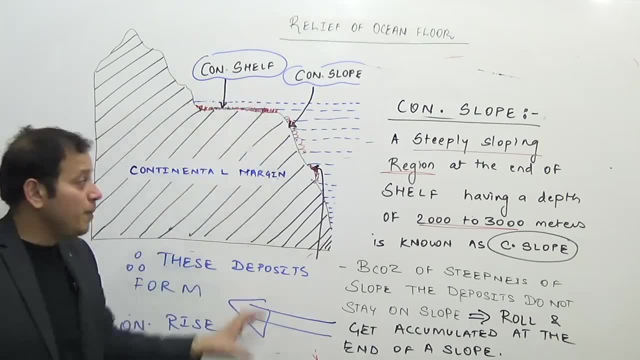 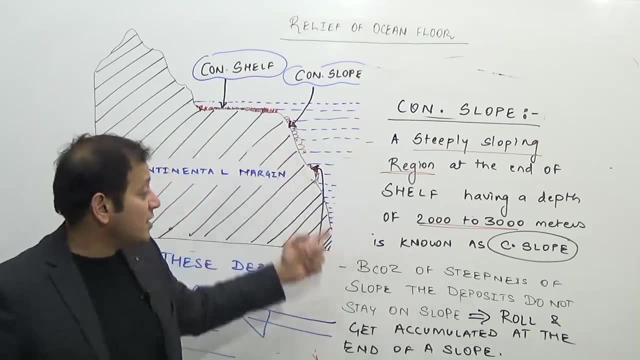 So this is what is the continental shelf, continental slope and continental rise. Again, continental rise may be there or may not be there, because if it is very, if there is sudden, suddenly at the end of a slope there is a trench, then obviously the deposits.